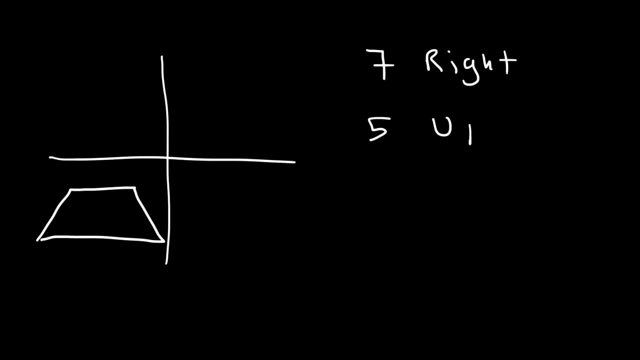 And let's say, 5 units up. So we're going to have to travel 5 units up And then 7 units to the right. So most likely the graph will be in quadrant 1.. So that's the main idea behind translation. 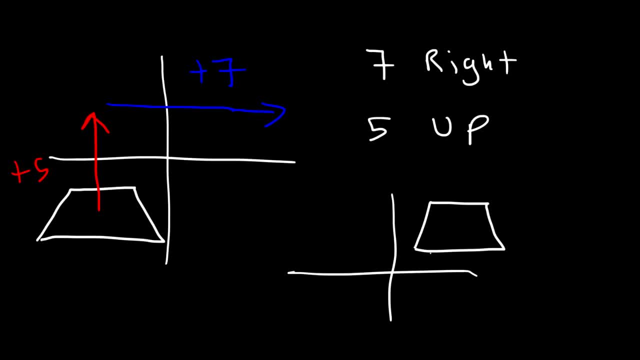 So, basically, you're moving the same image either to the left, to the right, up or down a coordinate plane. But let me give you a specific example. So let's draw a graph first. Let's draw a graph first. Let's draw a graph first. 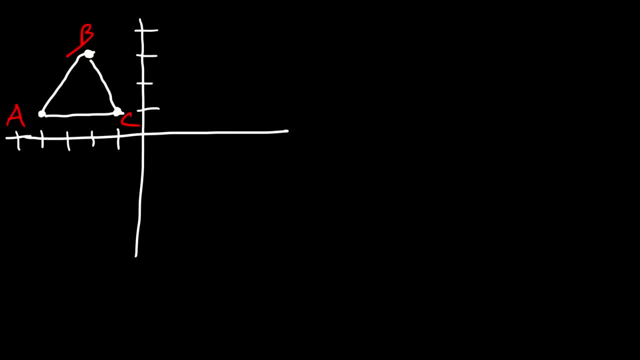 And point C. Translate the graph: 5 units to the right And 4 units down. So if you move it to the right it's going to be in quadrant 1. And then, if you move it down, most likely it's going to be in quadrant 3.. 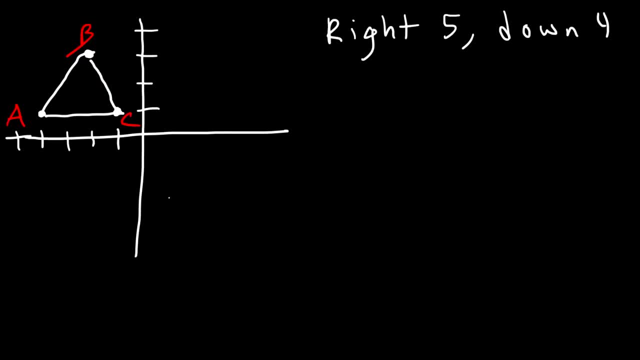 So, therefore, we should have some figure. I mean, this is quadrant 4,, by the way, We should have some figure in quadrant 4.. That looks like this: It should have the same size, but in a different position. Now, the best way to go about doing this is to find all the points of the original figure. 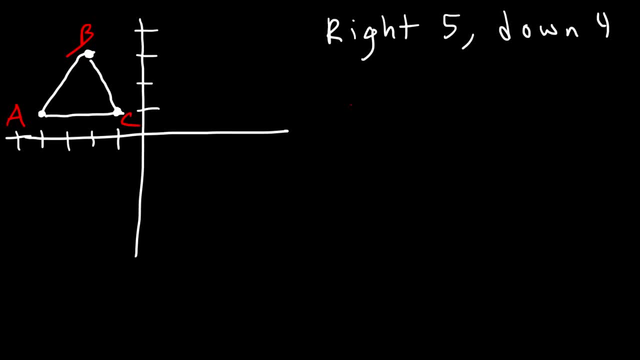 So point A: if you look at the graph carefully, point A is at negative 4, comma 1.. Point B: Point B is located at negative 2.. I'm going to say it's closer to negative 2 than negative 3.. 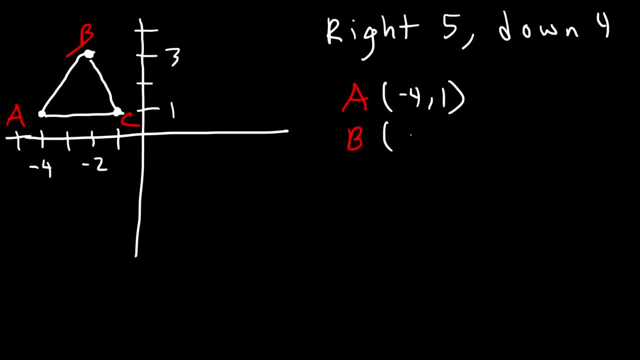 And it has a y value of 3.. And then point C is located at negative 1, comma 1.. So that's for the original figure. Now, to find the points of the new figure, we need to add 5 to the x values, because the graph is going to be shifted 5 units to the right. 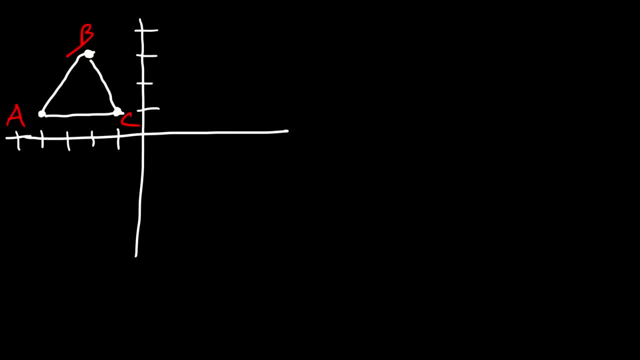 And point C. Translate the graph: 5 units to the right And 4 units down. So if you move it to the right it's going to be in quadrant 1. And then, if you move it down, most likely it's going to be in quadrant 3.. 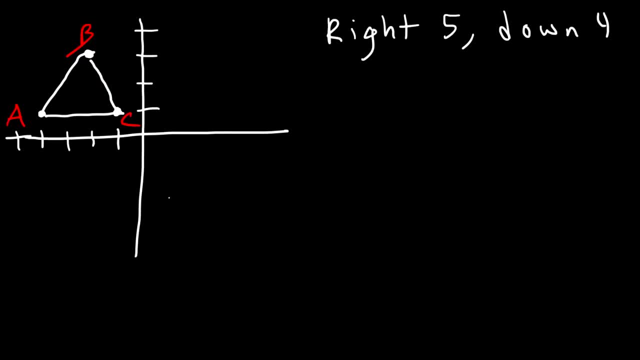 So, therefore, we should have some figure. I mean, this is quadrant 4,, by the way, We should have some figure in quadrant 4.. That looks like this: It should have the same size, but in a different position. Now, the best way to go about doing this is to find all the points of the original figure. 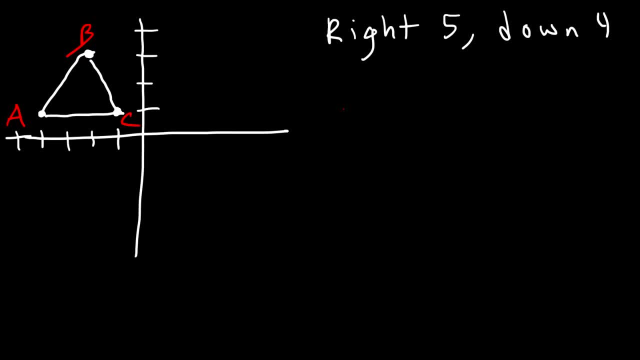 So point A: if you look at the graph carefully, point A is at negative 4, comma 1.. Point B: Point B is located at negative 2.. I'm going to say it's closer to negative 2 than negative 3.. 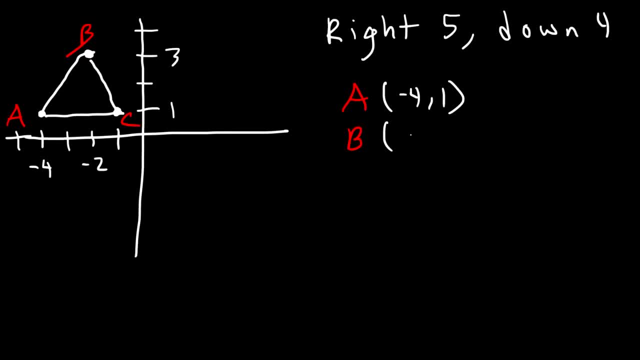 And it has a y value of 3.. And then point C is located at negative 1, comma 1.. So that's for the original figure. Now, to find the points of the new figure, we need to add 5 to the x values, because the graph is going to be shifted 5 units to the right. 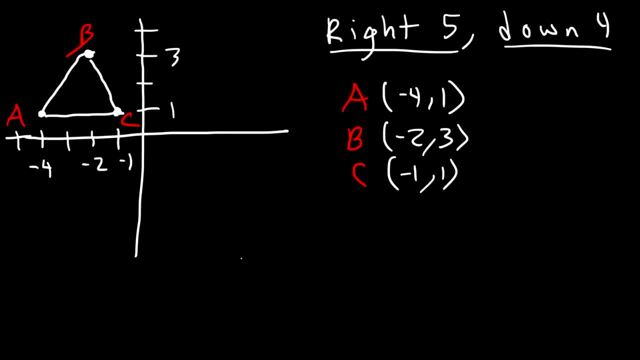 And then we need to subtract 4 from the y values. So this is the original point A. It's negative 4, comma 1.. And then we're going to add 5 to the x values and then subtract the y values by 4.. 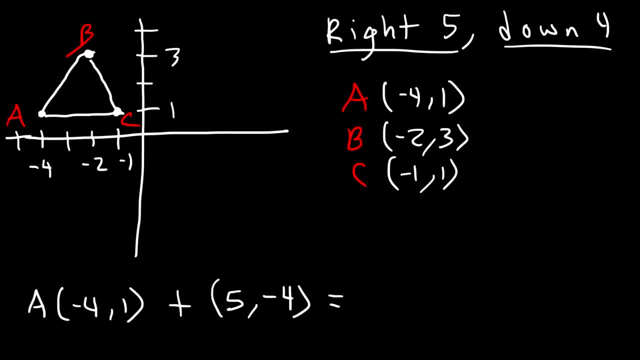 So negative. 4 plus 5. Is 1. 1 minus 4 is negative 3. So the new coordinates for A are: 1, comma, negative 3.. Now let's do the same for B. So B is at negative 2, comma 3.. 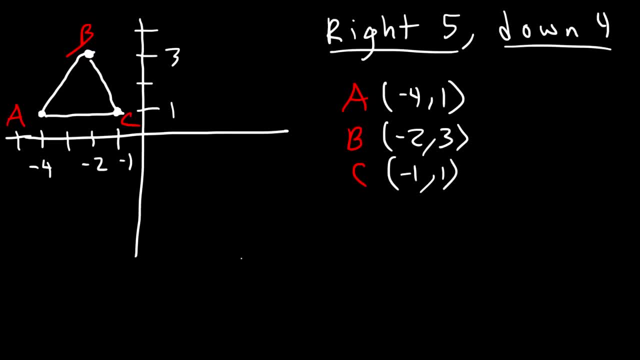 And then we need to subtract 4 from the y values. So this is the original point A. It's negative 4, comma 1.. And then we're going to add 5 to the x values and then subtract the y values by 4.. 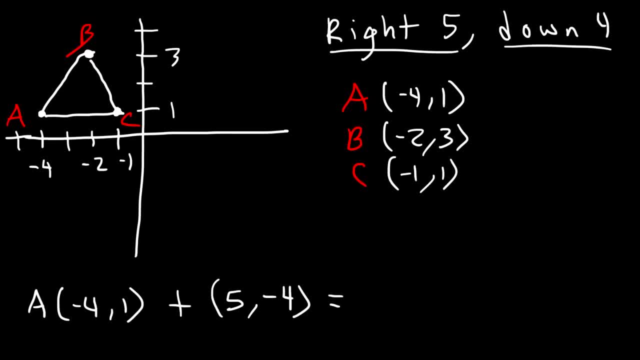 So negative. 4 plus 5. Is 1. 1 minus 4 is negative 3. So the new coordinates for A are: 1, comma, negative 3.. Now let's do the same for B. So B is at negative 2, comma 3.. 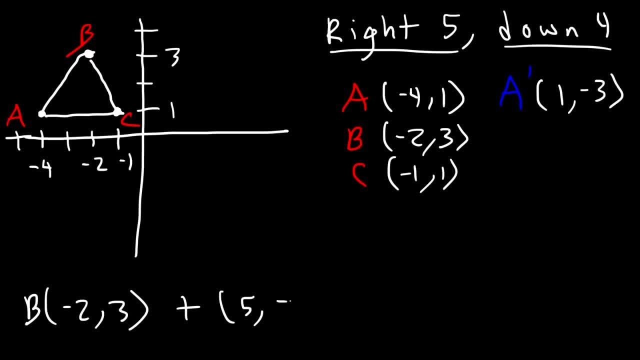 And then we're going to add 5 to the x coordinate and subtract the y coordinate by 4.. Negative 2 plus 5 is 3. And 3 minus 4 is negative 1.. So this is the new coordinates for B. 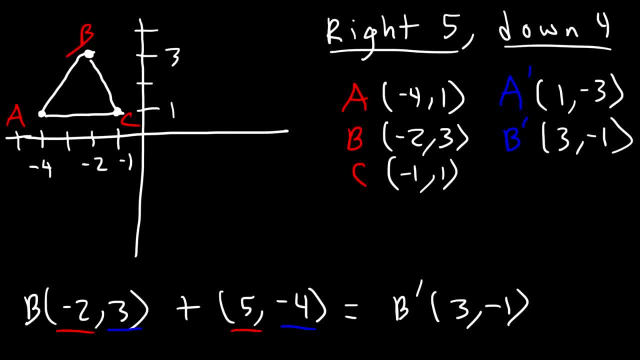 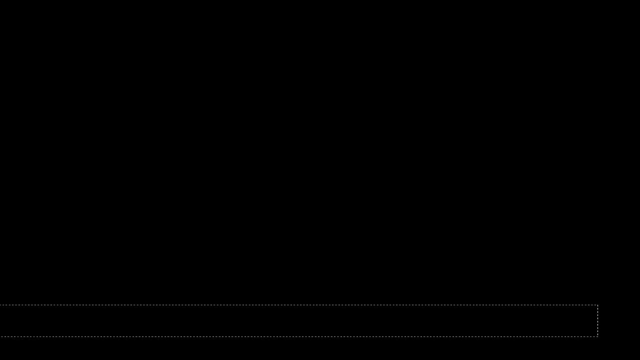 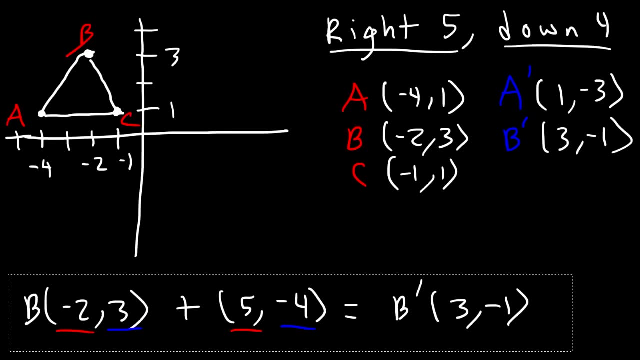 It's 3, comma, negative 1.. Now let's follow the same procedure. Okay, what just happened? Let's follow the same procedure for point C: Negative 1 plus 5. is 4.. And then, if we add 1 and negative 4,, 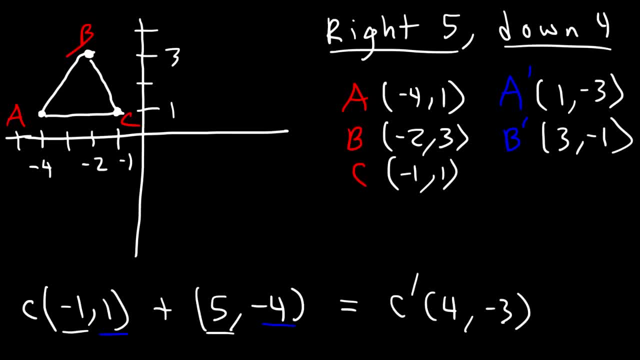 that's going to be negative 3.. So the new point for C is located at 4, negative 3.. So now all we need to do is plot the new points for A, B and C, And then we can graph a figure. 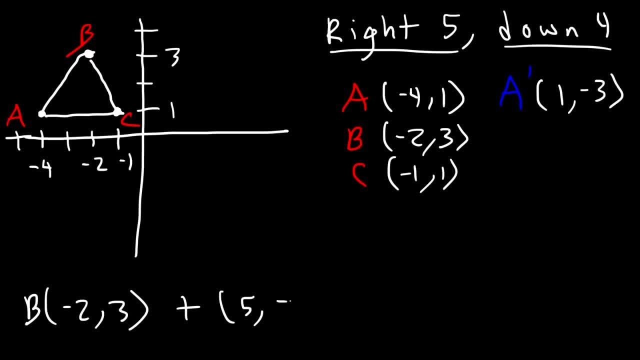 And then we're going to add 5 to the x coordinate and subtract the y coordinate by 4.. Negative 2 plus 5 is 3. And 3 minus 4 is negative 1.. So this is the new coordinates for B. 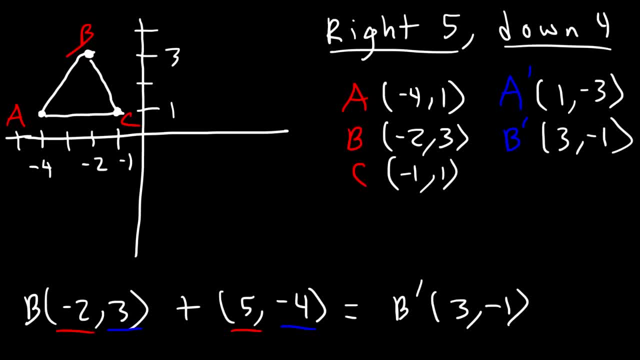 It's 3, comma negative 1.. And then we're going to add 5 to the x coordinate and subtract the y coordinate by 4.. And then we're going to add 5 to the x coordinate and subtract the y coordinate by 4.. 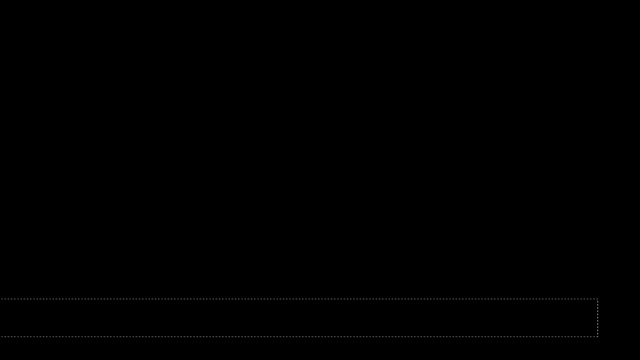 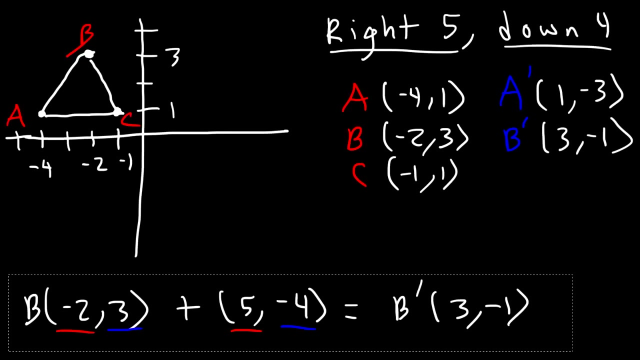 Now let's follow the same procedure. Okay, what just happened? Let's follow the same procedure for point C. Let's follow the same procedure for point C. Negative 1 plus 5. Is 4.. And then if we add 1 and negative 4, that's going to be negative 3.. 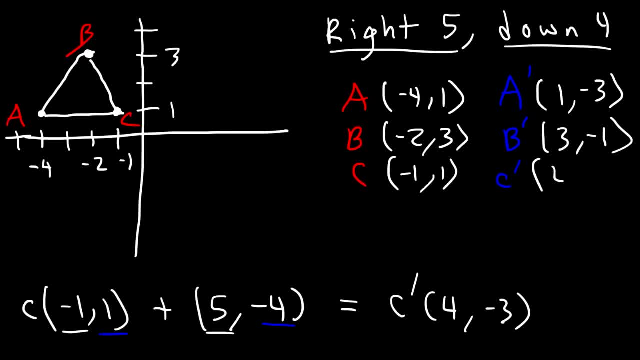 So the new point for C is located at 4, comma, negative 3.. So now all we need to do is plot the new points for A, B and C And then we can graph a figure. So point A is located at 1, negative 3,, which is here: 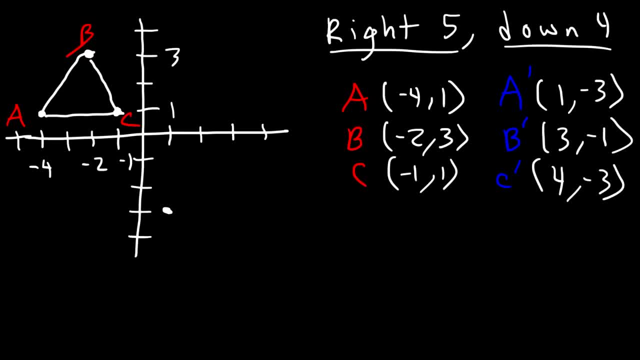 And then point B is located at 3, negative 1.. And C is located at 4, negative 3.. And then point A is located at 4, negative 3.. So, as you can see, we shifted the graph 5 units to the right and then 4 units down. 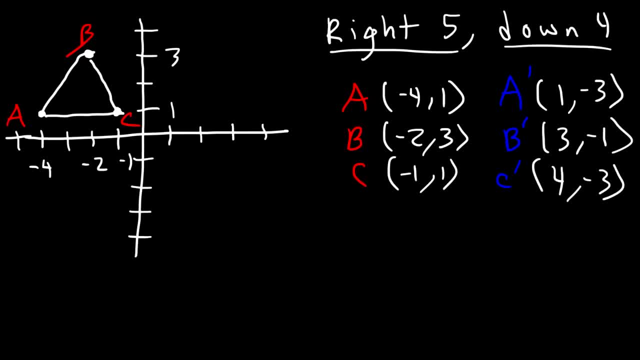 So point A is located at 1, negative 3, which is here, And then point B is located at 3, negative 1.. And C is located at 4, negative 3.. So, as you can see, we shifted the graph 5 units to the right. 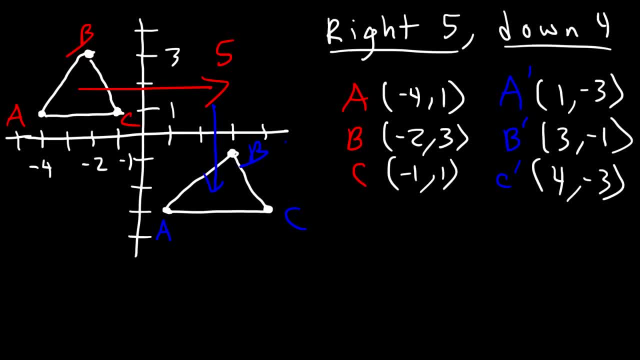 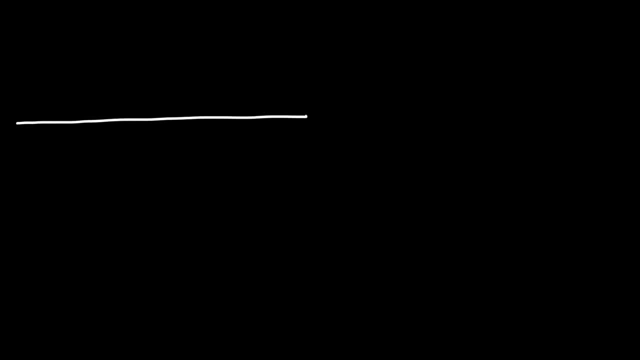 and then 4 units down, And so it should be in this quadrant. For the sake of practice, let's try another example. So let's say this is point A, B, C and D. What I want you to do is pause the video. 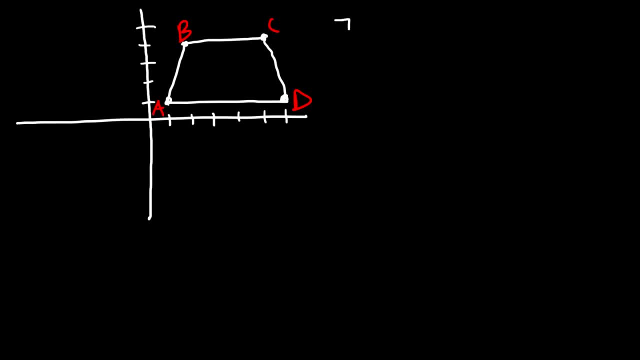 and shift the graph 7 units to the left and 6 units down. So follow the same process And then, once you're ready, once you finish it, unpause the video to see if you have the right answer. So the first thing we need to do is identify. 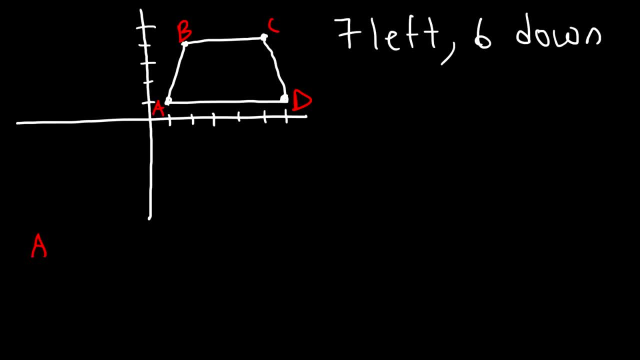 all of the original points. So point A is located at 1, 1.. Point B is located at 2, 4.. Point C is located at 5, 4. And point D is located at 6, 1.. 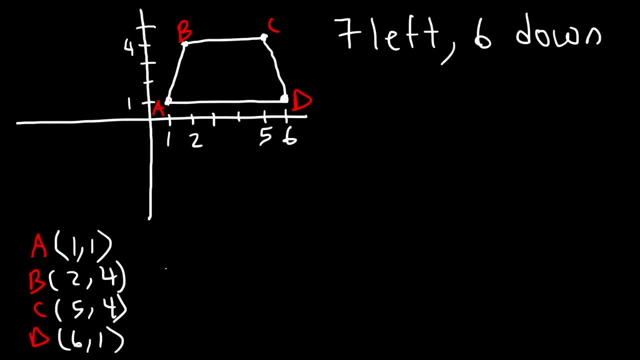 So now to each of these points, we need to travel 7 units to the left. So therefore we're going to subtract the x values by 7, or just add negative 7 to it, And now we need to go down 6 units. 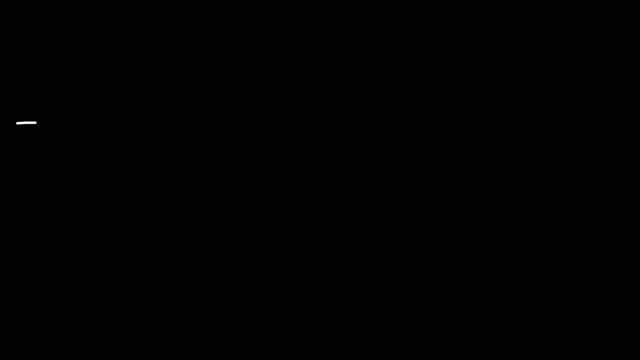 And so it should be in this quadrant. For the sake of practice, let's try another example. So let's say this is point A, B, C and D. What I want you to do is pause the video and shift the graph 7 units to the left and 6 units down. 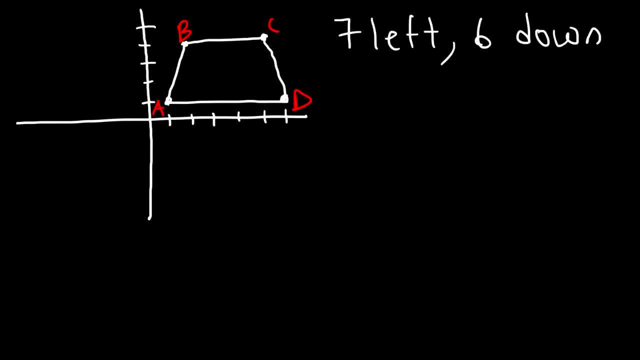 So follow the same process and then, once you're ready, once you finish it, unpause the video to see if you have the right answer. So the first thing we need to do is identify all of the original points. So point A is located at 1, 1.. 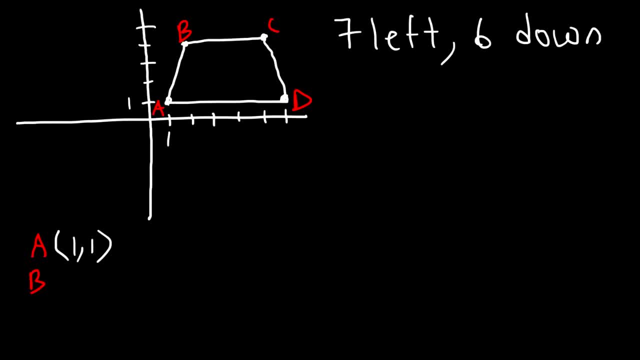 Okay, Point B is located at 2, 4.. Point C is located at 5, 4. And point D is located at 6, 1.. So now to each of these points. we need to travel 7 units down. 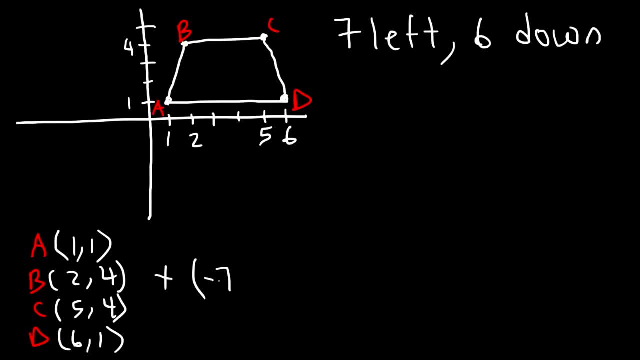 7 units to the left. So therefore we're going to subtract the x values by 7 or just add negative 7 to it, And now we need to go down 6 units, So we've got to decrease the y values by 6.. 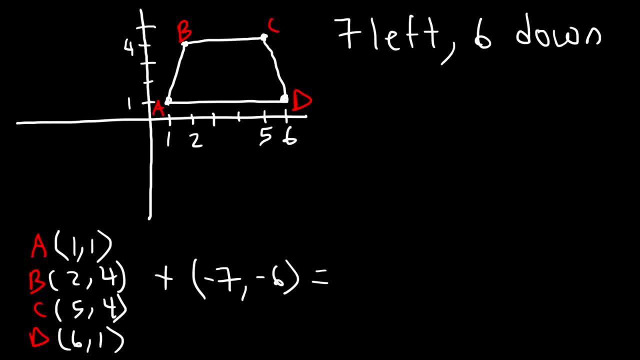 So we've got to add negative 6 to it. So let's start with the x values. 1 plus negative 7 is negative. 6, 2 plus negative 7 is negative. 5, 5 plus negative 7 is negative. 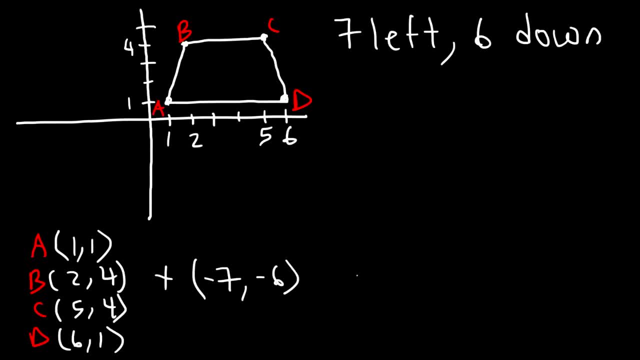 So we've got to decrease the y values by 6.. So we've got to add negative 6 to it. So let's start with the x values. 1 plus negative 7 is negative 6.. 2. 2 plus negative 7 is negative 5.. 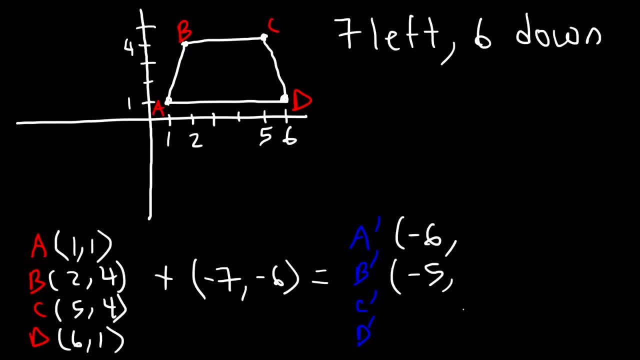 5 plus negative- 7 is negative 2.. And 6 plus negative 7 is negative 1.. So now let's focus on the y values: 1 plus negative 6, that's going to be negative 5.. And then 4 plus negative- 6 is negative 2.. 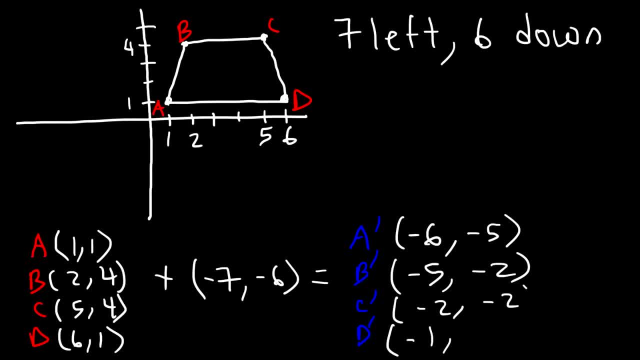 And 4 plus negative 6 is negative 2.. Well, that's going to be the same. So B and C has the same y value And 1 plus negative 6 is negative 5, just like point A is. So now that we have the new points for the translated image, 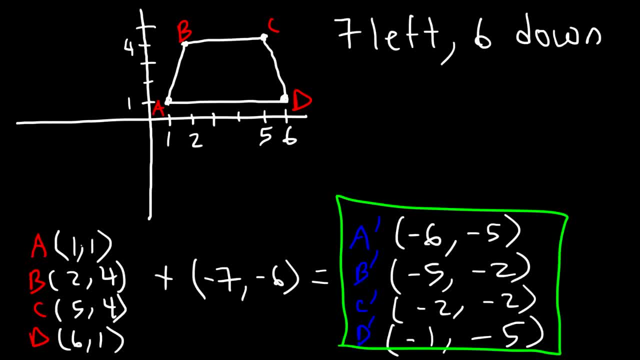 let's go ahead and plot those points. So the new point for A is at negative 6, negative 5.. So that's somewhere in this region. And then B is now at negative 5, negative 2.. C is at negative 2, negative 2.. 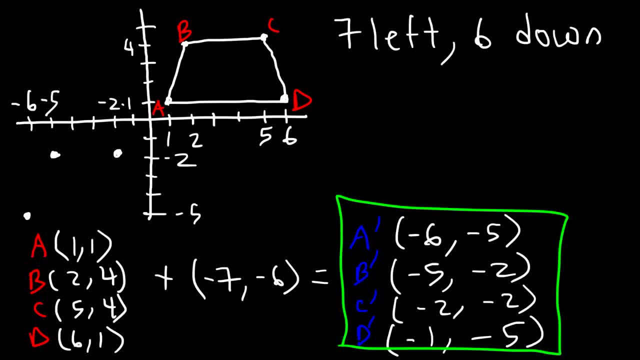 And D is located at negative 1, negative 5.. So this is the new point for A, B, C and D. So we traveled 7 units to the left And then we traveled down 6 units. So that moves the quadrilateral from quadrant 1.. 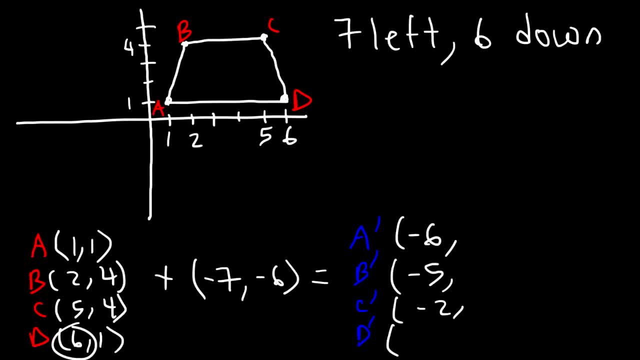 2, and 6 plus negative: 7 is negative 1.. So now let's focus on the y values: 1 plus negative 6. That's going to be negative 5.. And then 4 plus negative 6 is negative 2.. 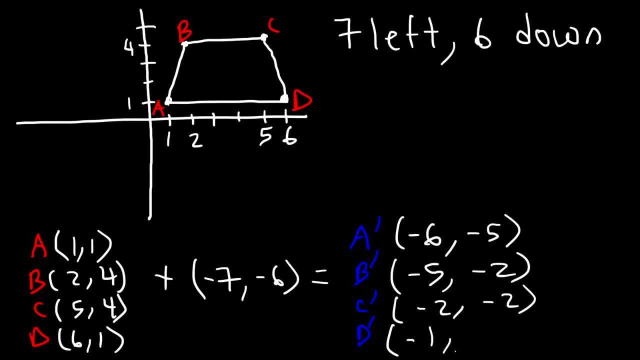 And 4,. well, that's going to be the same. So B and C has the same y value And 1 plus negative 6 is negative 5, just like point A is. So now that we have the new points for the translated image, let's go ahead and plot. 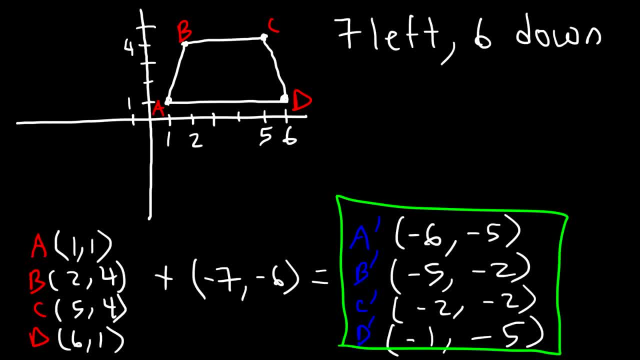 those points. Okay, Okay, Okay. So the new point for A is at negative 6, negative 5.. So that's somewhere in this region. And then B is now at negative 5, negative 2.. Okay, Okay. 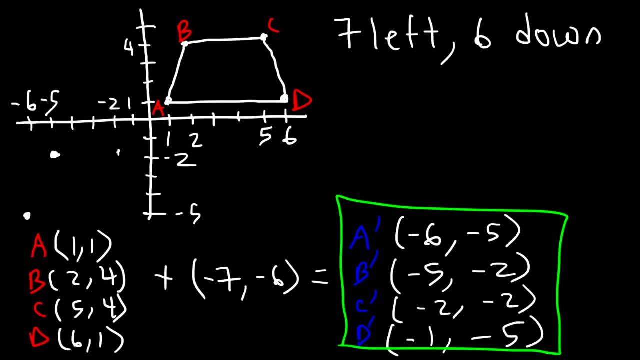 So B is at negative 2, negative 2.. And D is located at negative 1, negative 5.. So this is the new point for A, B, C and D. So we traveled 7 units to the left. 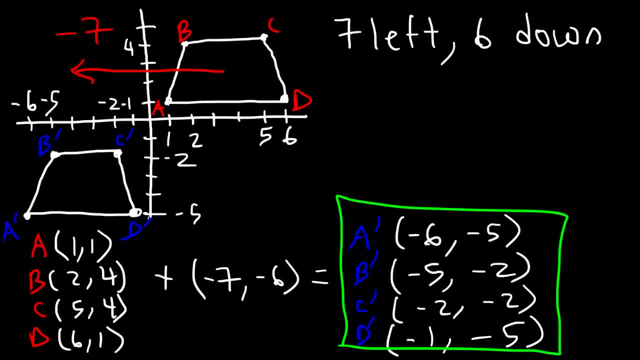 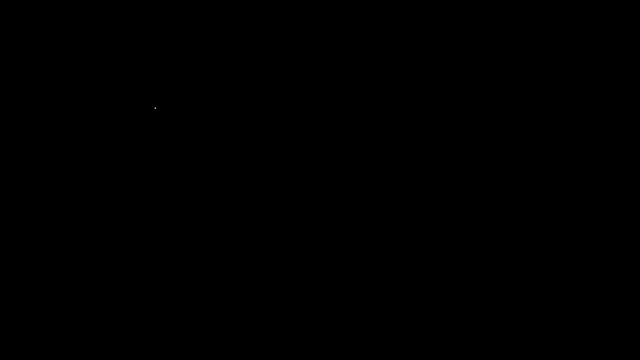 And then we traveled down 6 units, So that moves the quadrilateral from quadrant 1 to quadrant 3.. Now let's talk about reflections. There's three reflections that you may need to know: A reflection over the x-axis, over the y-axis and over the origin. 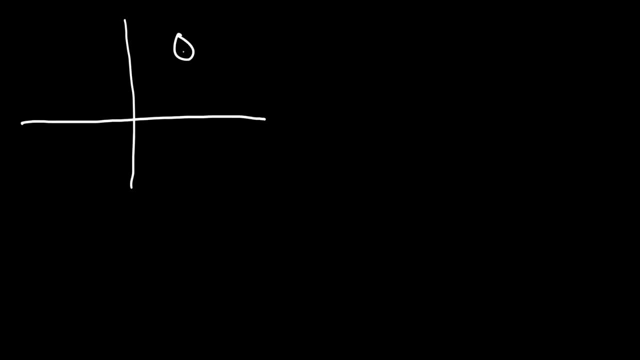 By the way, You may not be familiar with quadrants. This is quadrant 1,, where x and y are both positive. In quadrant 2, x is negative, y is positive, And this is quadrant 3, where both x and y are negative. 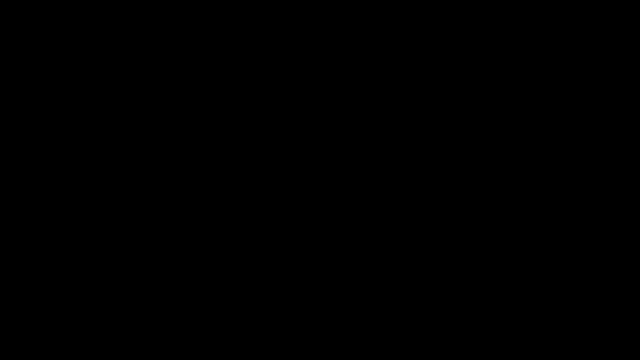 So that moves the quadrilateral from quadrant 1.. So that moves the quadrilateral from quadrant 1 to quadrant 3.. Now let's talk about reflections. There's three reflections that you may need to know: A reflection over the x-axis, over the y-axis and over the origin. 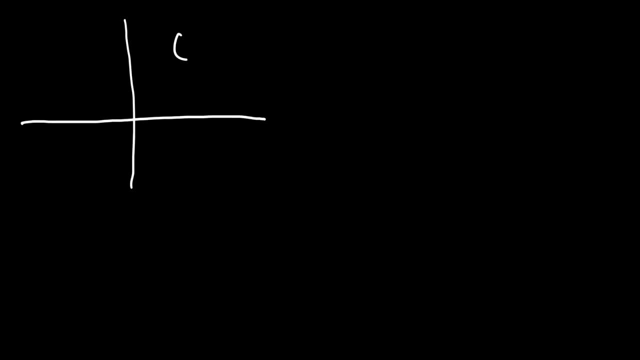 By the way, for those of you who may not be familiar with quadrants, this is quadrant 1, where x and y are both positive. In quadrant 2, x is negative, y is positive, And this is quadrant 3, where both are positive. 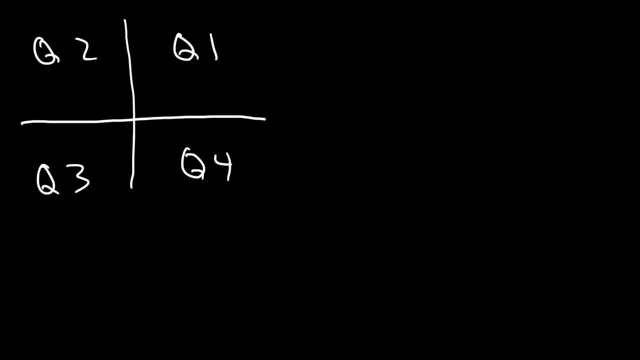 Both x and y are negative. And in quadrant 4, x is positive, y is negative. So let's say, if we have a triangle in quadrant 1. And we wish to reflect this triangle over the x-axis. So this is the x-axis and here is the y-axis. 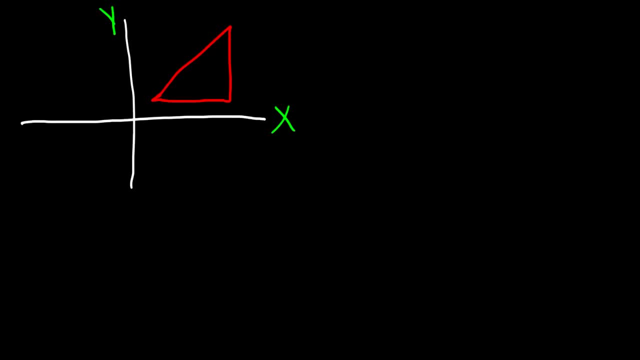 How will the image look? How can we draw If you're going to reflect something over the x-axis? it's going to move from quadrant 1 to quadrant 4. And it's going to flip at the same time. So the new image is going to look like this. 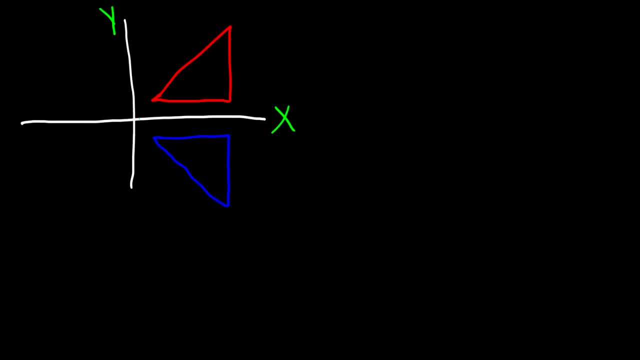 As you can see, the x-axis is basically the line of symmetry. The blue triangle is basically a reflection or a mirror image of the red triangle, Where the x-axis? you can think of it as the mirror Or the line of symmetry. 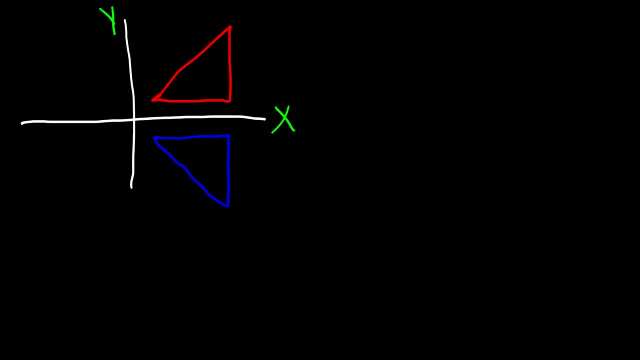 So that's how you can reflect an image over the x-axis. So let me give you another example. So let's say, if we have a trapezoid in quadrant 2. And we wish to reflect it over the x-axis, So all you've got to do is you need to move the trapezoid to quadrant 3.. 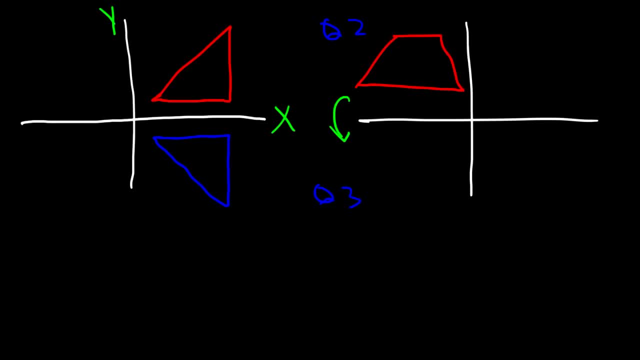 It's going to move from Quadrant 2 to quadrant 3.. And then you need to flip it, So notice that the long side is closer to the x-axis. When you draw it in quadrant 3, the long side will still be closer to the x-axis. 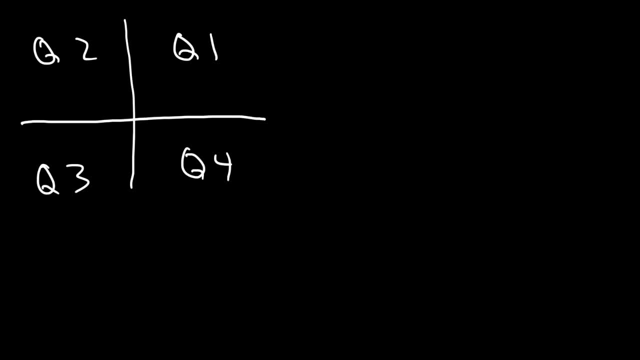 And in quadrant 4, x is positive, y is negative. So let's say, if we have a triangle in quadrant 1, and we wish to reflect this triangle over the x-axis, So this is the x-axis and here is the y-axis. 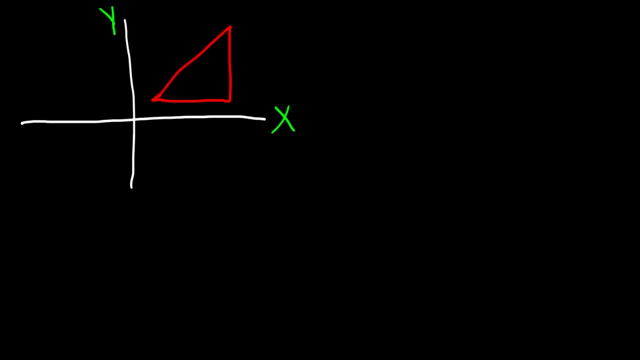 How will the image look? How can we draw If you can reflect something over the x-axis? it's going to move from quadrant 1 to quadrant 4. And it's going to flip at the same time. So the new image is going to look like this. 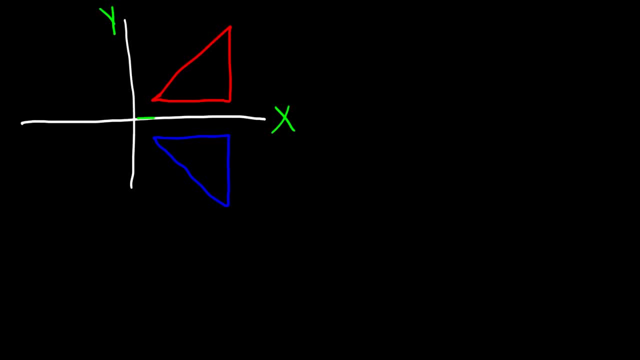 As you can see, The x-axis is basically the line of symmetry. Okay, The blue line, I mean the blue triangle, is basically a reflection or a mirror image of the red triangle, Where the x-axis- you can think of it as the mirror. 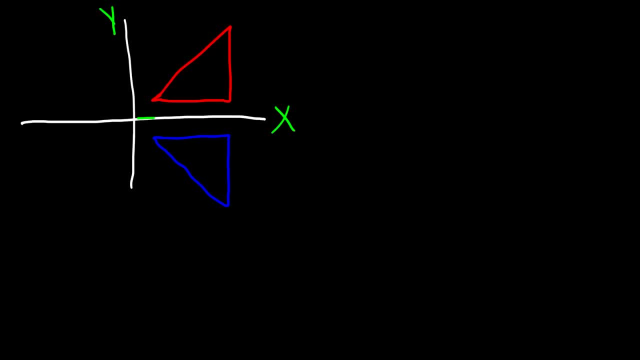 Or the line of symmetry. So that's how you can reflect an image over the x-axis. So let me give you another example. So let's say, if we have a trapezoid In quadrant 2. And we wish to reflect it over the x-axis, 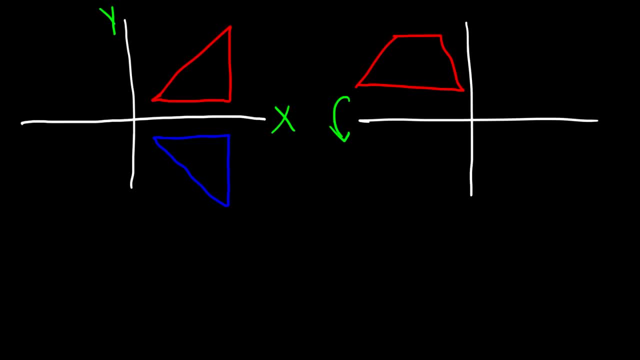 So all you got to do is you need to move the trapezoid to quadrant 3.. It's going to move from quadrant 2 to quadrant 3.. And then you need to flip it, So notice that the long side is closer to the x-axis. 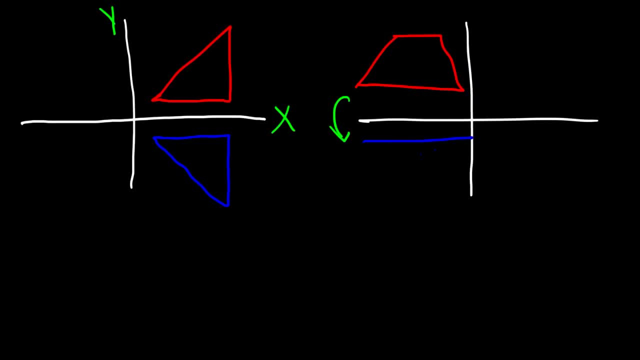 When you draw in quadrant 3, the long side will still be closer to the x-axis. This is the x-axis. Okay, It's going to have the same length. Okay, let me do that better. It's going to be just as long. 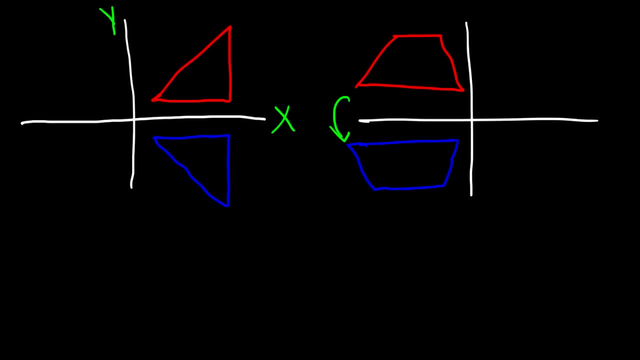 But it's just flipped over the x-axis, So my drawing's not perfect, but hopefully you get the picture Now. here's what you need to know. Anytime you want to reflect something over the x-axis, you need to multiply the y-coordinate. 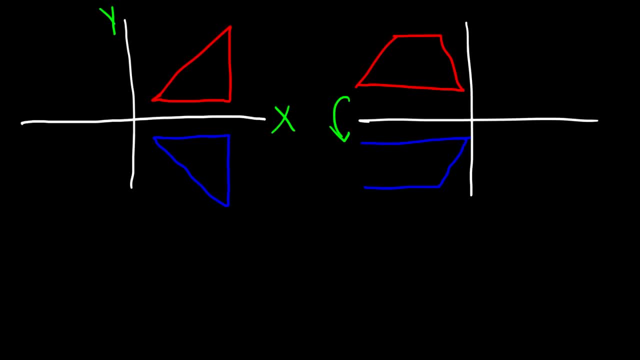 It's going to have the same length. Okay, let me do that better. It's going to be just as long, But it's just flipped over the x-axis. Okay, let's do this. My drawing's not perfect, but hopefully you get the picture. 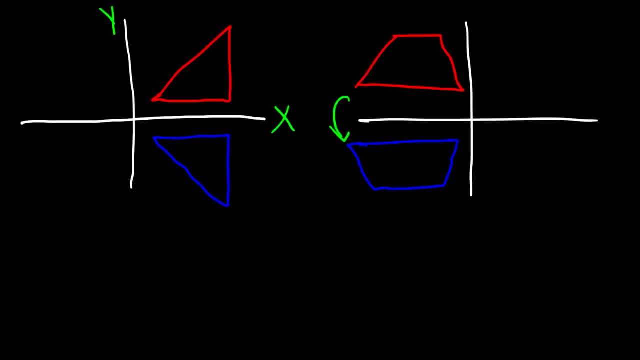 Now here's what you need to know: Anytime you want to reflect something over the x-axis, you need to multiply the y-coordinate by negative 1.. So in the first example, let's say we have some point, x, y. That new point is going to be located at x, negative y. 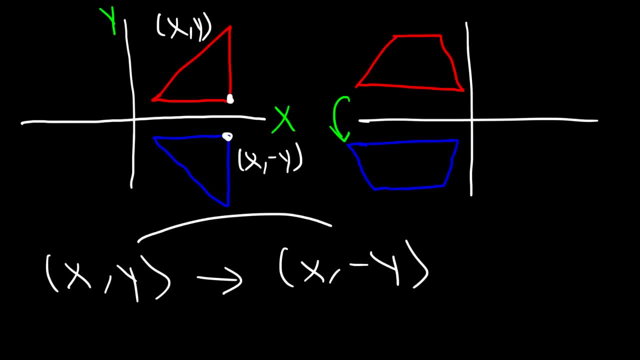 So all you've got to do is multiply The y-coordinate by negative 1.. That's how you can reflect it over the x-axis. Looking at the second example, let's focus on this point- It's in quadrant 2, so x is negative and y is positive. 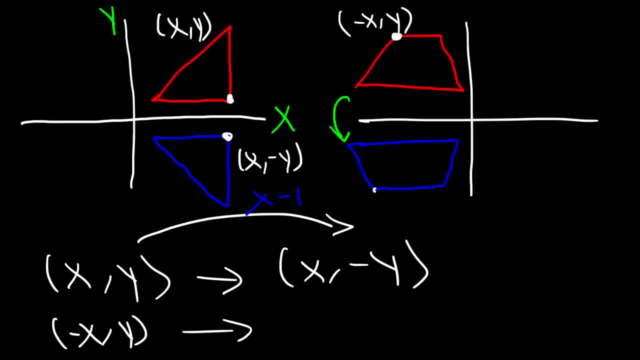 To reflect it over the x-axis, the new point will have the coordinates negative x, negative y. As you can see, this is still on the left side, so x is still negative- It's in quadrant 3, but y is negative in quadrant 3.. 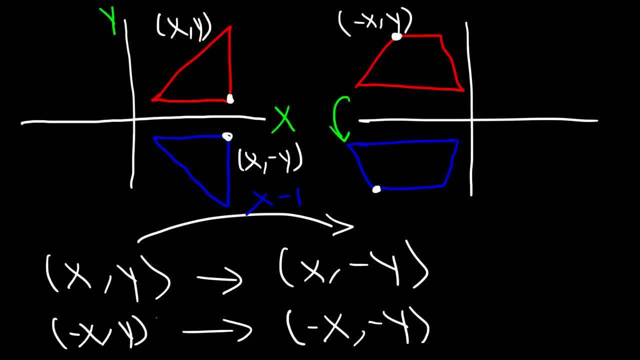 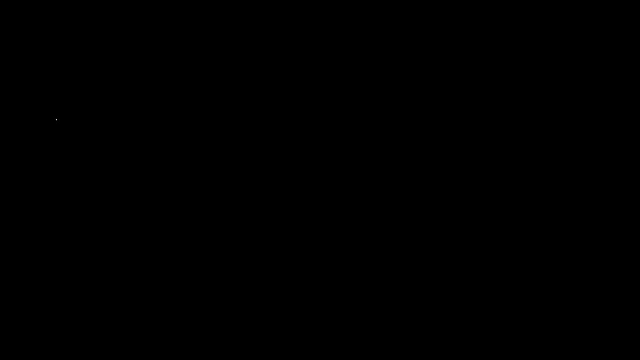 So the net effect is that we only change the y-coordinate. We're going to multiply the y-coordinate by negative: 1. The x-coordinate doesn't change when you're reflecting over the x-axis. Now let's talk about reflections over the y-axis. 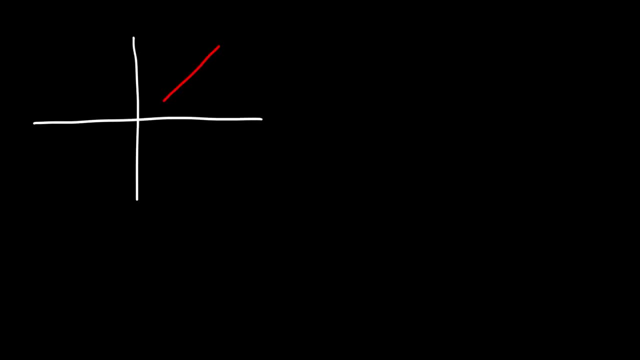 So let's start with our triangle again in quadrant 1.. So when you reflect it over the y-axis, it's going to flip over the y-axis, So you're going to get an image that looks like this. Now let's say, if you have some point, x, y, 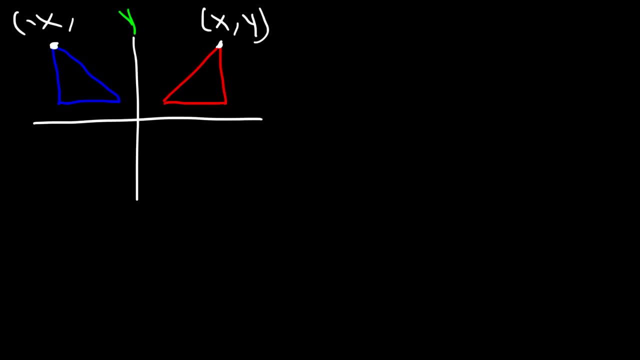 The new point will be negative x, y. So when you're reflecting over the y-axis, you need to multiply the x-coordinate by negative 1.. Let's look at another example. So let's say, if we have a trapezoid in quadrant 4,. 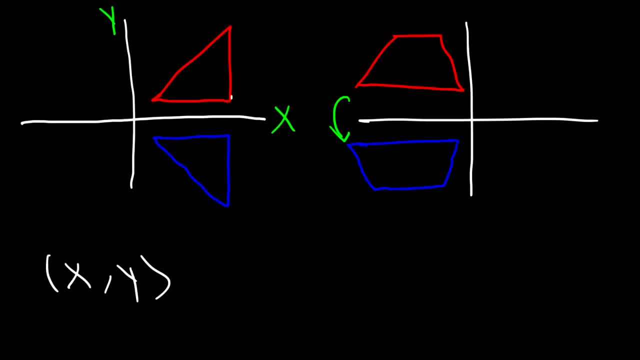 by negative 1.. So in the first example, Let's say we have some point xy. That new point is going to be located at x negative y. So all you got to do is multiply the y-coordinate by negative 1.. 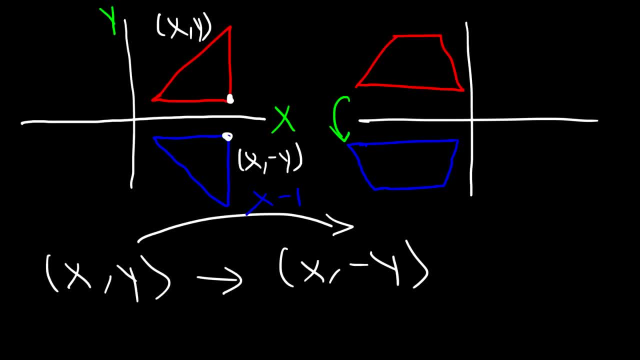 That's how you can reflect it over the x-axis. Looking at the second example, let's focus on this point. It's in quadrant 2, so x is negative and y is positive. Okay, To reflect it over the x-axis, the new point will have the coordinates negative, x, negative. 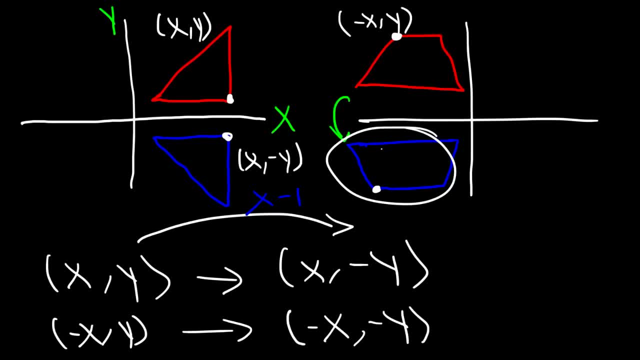 y. As you can see, this is still on the left side. so x is still negative, It's in quadrant 3, but y is negative in quadrant 3.. So the net effect is that we only change the y-coordinate. We're going to multiply the y-coordinate by negative 1.. 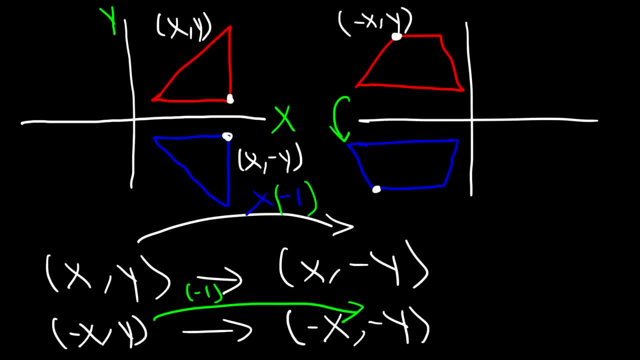 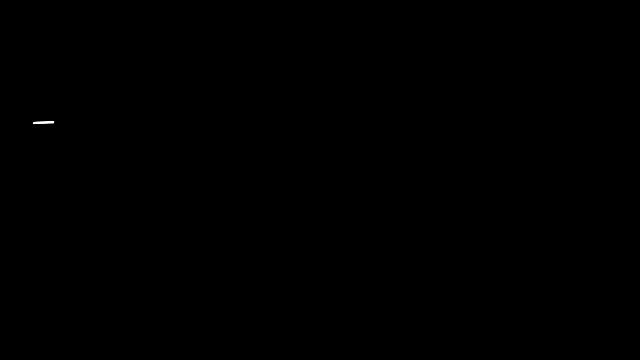 Okay, So that's it. The x-coordinate doesn't change when you're reflecting over the x-axis. Now let's talk about reflections over the y-axis. So let's start with our triangle again in quadrant 1.. So when you reflect it over the y-axis, it's going to flip over the y-axis. 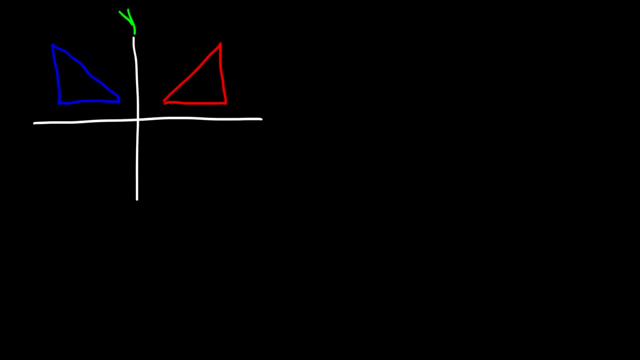 So you're going to get an image that looks like this: Okay, Okay, Okay, Okay. Now let's say if you have some point. The new point will be: So when you're reflecting over the y-axis, you need to multiply the x-coordinate by negative. 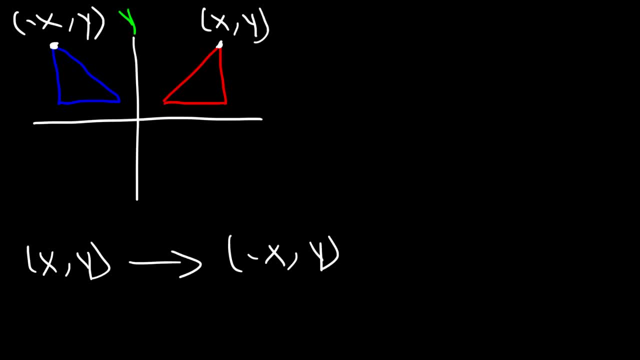 1. Let's look at another example. Okay, So let's say, if we have a trapezoid in quadrant 4, and we wish to reflect it over the y-axis, So it's going to move to quadrant 3.. 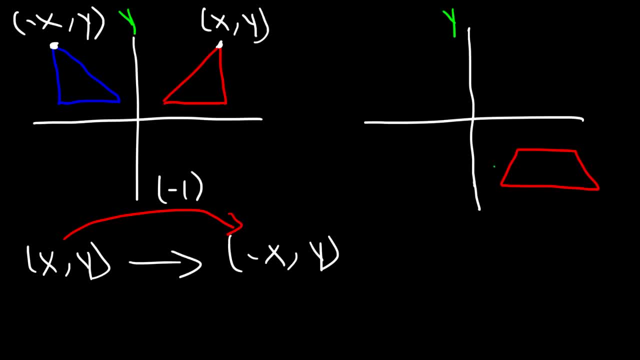 and we wish to reflect it over the y-axis, So it's going to move to quadrant 3.. So, therefore, you're going to get an image that looks like this, And that's basically it. So if we focus on a single point in quadrant 4,, 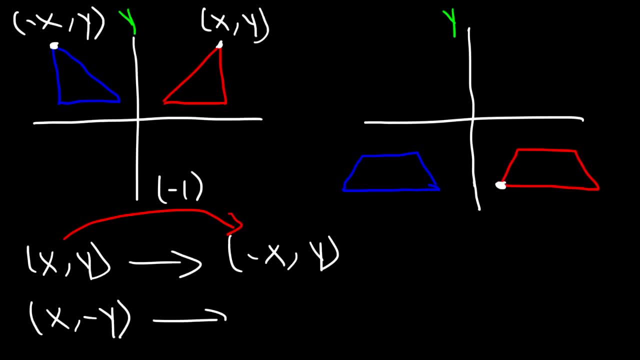 x is positive, y is negative And when we reflect it over the y-axis, multiply x by negative 1. So it becomes negative x, negative y, Which in quadrant 3, x and y are both negative. So to review what we just went over, 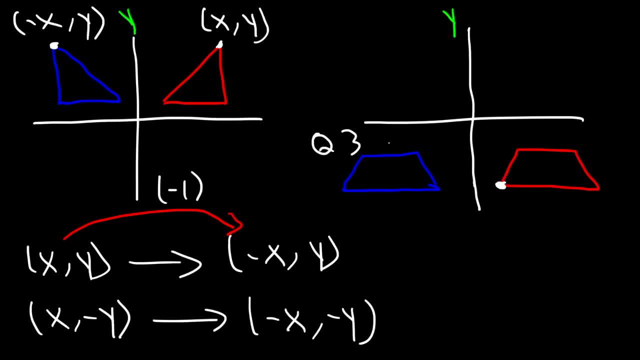 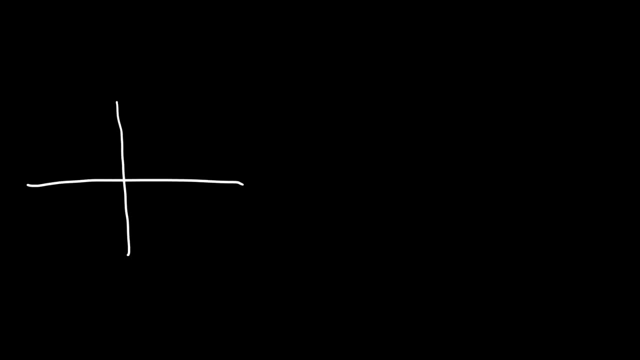 any time. you wish to reflect a figure over the x-axis, multiply the y-coordinate by negative 1.. If you wish to reflect it over the y-axis, multiply the x-coordinate by negative 1.. Now the next thing that we need to talk about is reflection over the origin. 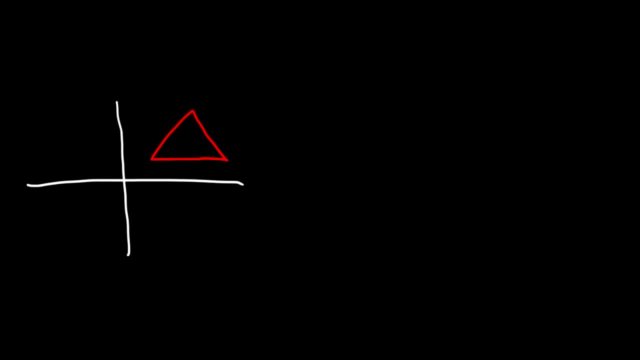 So let's say if we have a triangle in quadrant 1.. What's going to happen if we reflect it over the origin? So, to reflect it over the origin, it's going to move from quadrant 1 to quadrant 3.. Reflection about the origin is equivalent to reflecting it over the x-axis and then the y-axis. 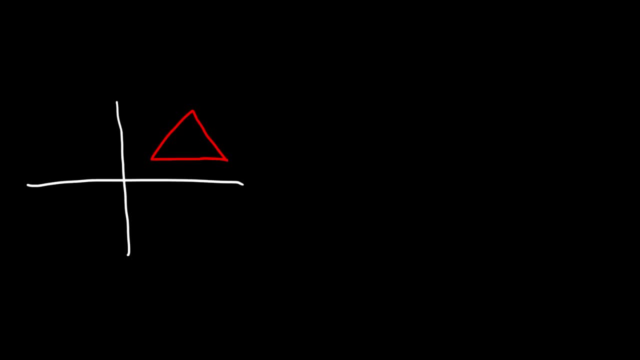 Or it could be over the y-axis first and then the x-axis. So if we reflect it over the y-axis, the graph will look like this: And then, if we reflect the green triangle over the x-axis, it's going to look like this: 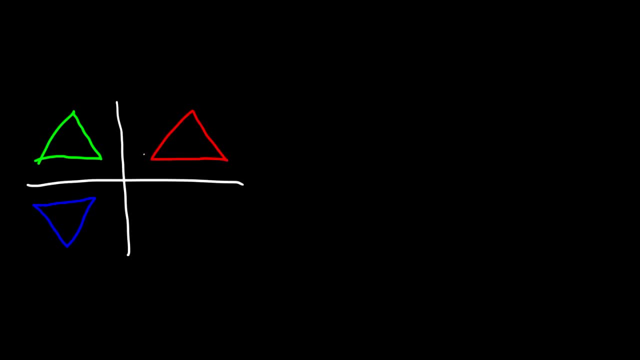 So going from red to blue. that's a reflection about the origin. Now, if we want to reflect it over the x-axis, first it's going to look like this And then, if we reflect it over the y-axis, it's going to move from quadrant 4 to quadrant 2,. 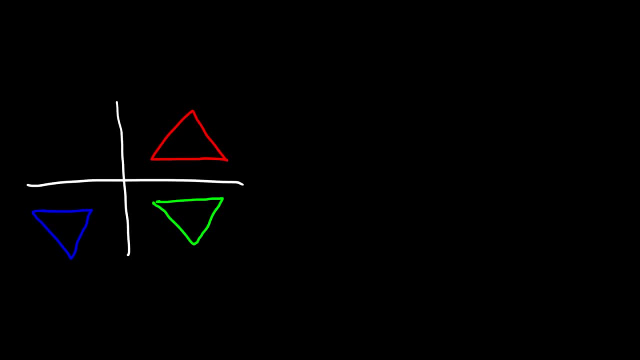 and it's going to be the same image, So the order doesn't matter. Now, when you want to reflect an image or figure from or about the origin, you need to multiply the x and the y value by negative 1.. So this is going to change to negative x, negative 1.. 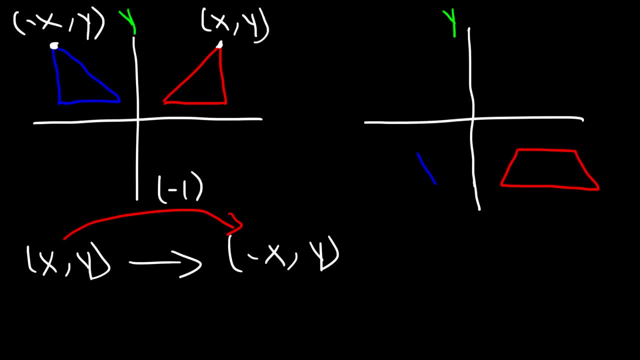 So, therefore, you're going to get an image that looks like this: Okay, So that's basically it. So, if we focus on a single point in quadrant 4, x is positive, y is negative, And when we reflect it over the y-axis, multiply x by negative 1.. 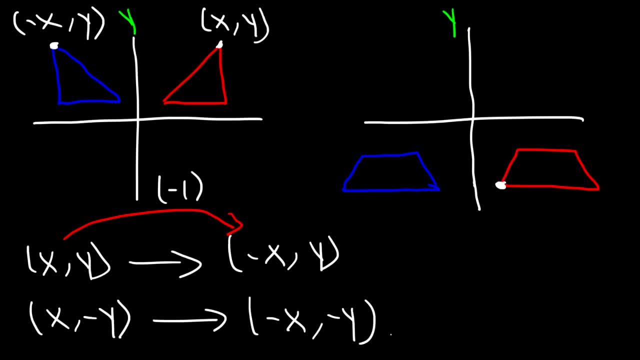 So it becomes negative x, negative y, which, in quadrant 3, x and y are both negative. So to review what we just went over, Anytime you wish to reflect a figure over the x-axis, multiply the y-coordinate by negative 1.. 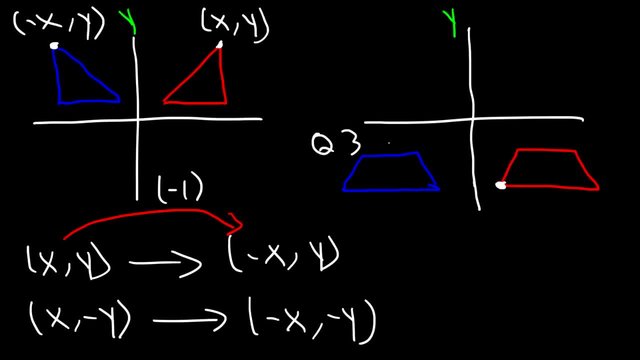 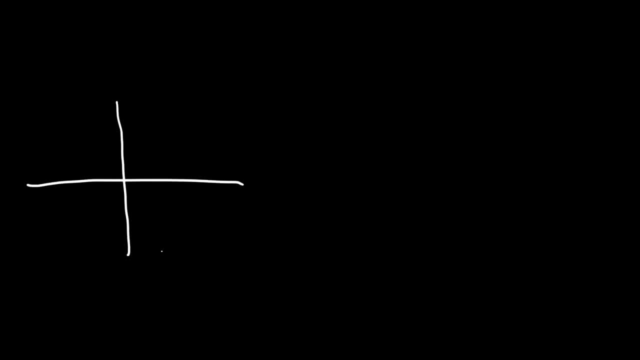 If you wish to reflect it over the y-axis, multiply the x-coordinate by negative 1.. Now the next thing that we need to talk about is a reflection over the origin. So let's say, if we have a triangle in quadrant 1.. 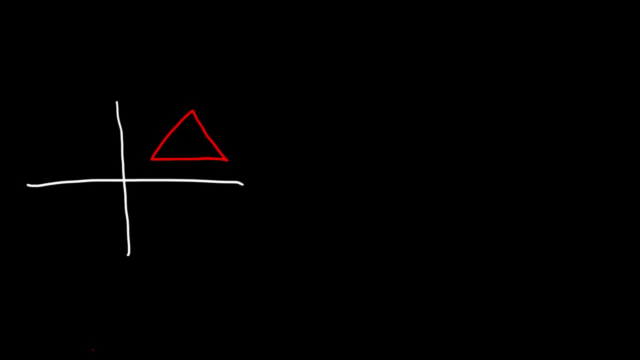 What's going to happen if we reflect it over the origin? Okay, So to reflect it over the origin, it's going to move from quadrant 1 to quadrant 3.. Reflection about the origin is equivalent to reflecting it over the x-axis and then 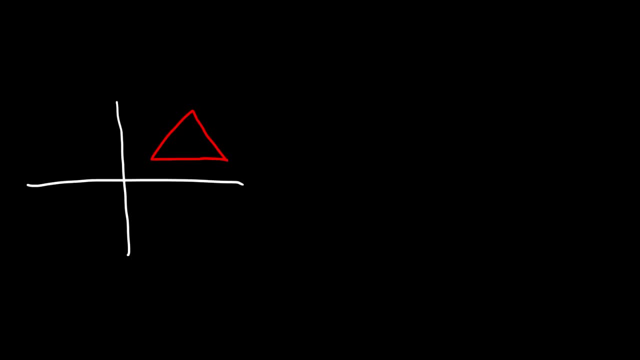 the y-axis, Or it could be over the y-axis first and then the x-axis. So if we reflect it over the y-axis, the graph will look like this: And then if we reflect the green triangle over the x-axis: Okay, 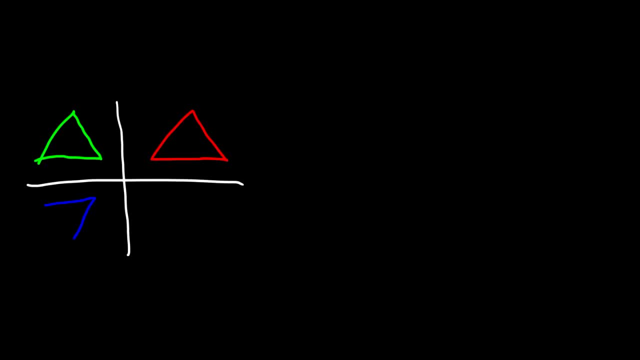 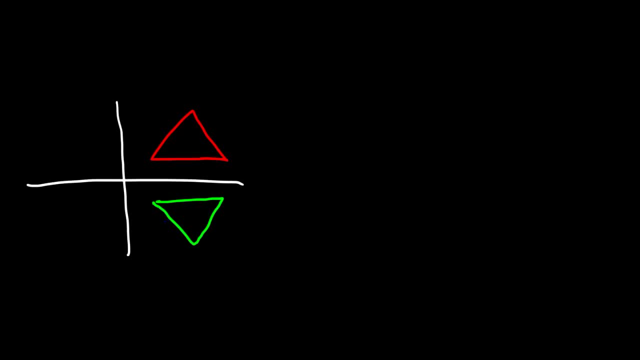 And then, if we reflect it over the y-axis, it's going to move from quadrant 4 to quadrant 2. And it's going to be the same image. So the order doesn't matter. Now, when you want to reflect in the x-axis, you're going to want to reflect over the y-axis. 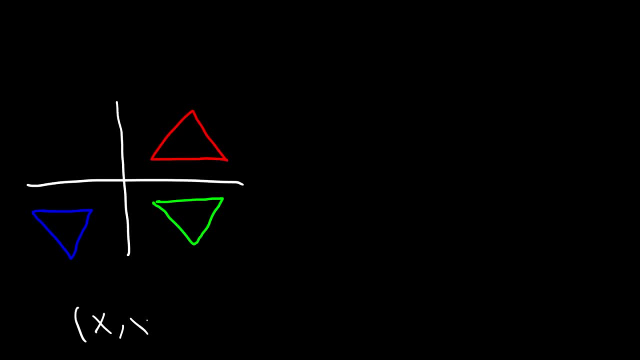 So if you want to reflect an image or figure from or about the origin, you need to multiply the x and the y value by negative 1.. So this is going to change to negative x, negative 1.. So here's another example. 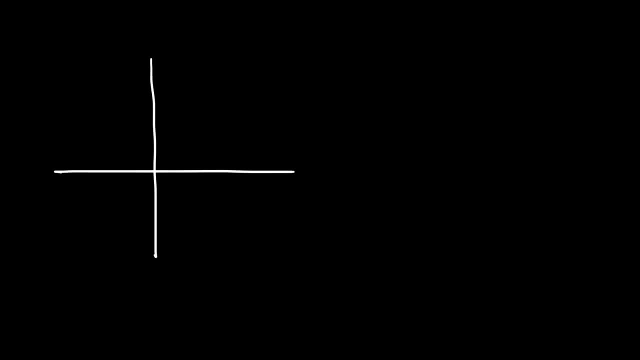 So here's another example. Let's say if we have a figure that looks like this and it's in quadrant 2.. Draw a rough sketch of the image after reflection about the origin. So it's going to move from quadrant 2 to quadrant 4.. 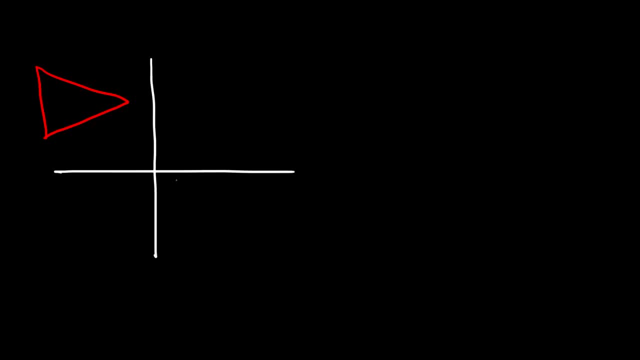 So if we reflect it about the y-axis first, it's going to look something like that, And then, if we reflect it over the x-axis, it's going to look like this. So basically, the blue image is a reflection of the red image about the origin. 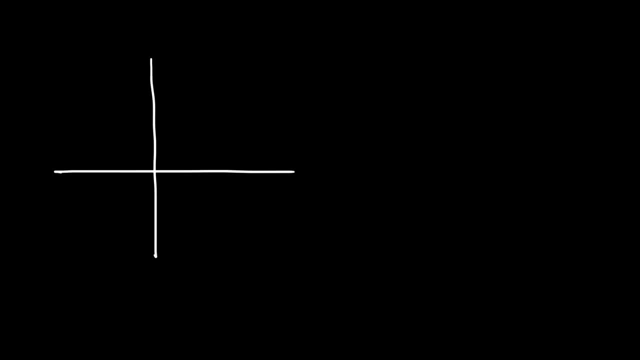 Now let me change the structure. Let's say, if we have a shape, an unusually looking shape like this, Let me make sure that one side is smaller relative to the other side. Reflect that image about the origin. So let's reflect it about the y-axis first. 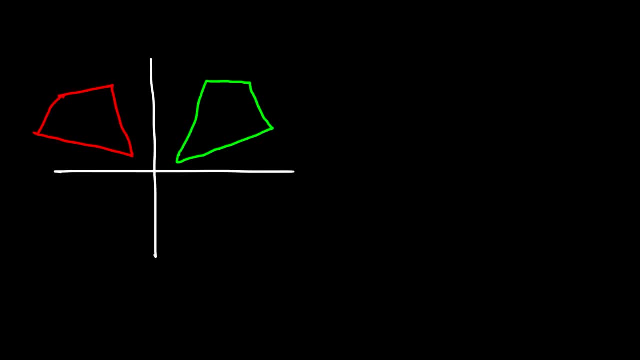 It's going to look something like that. And then, if we reflect it about the x-axis, it's going to look something like this. So this, the red one, is a reflection of the blue one about the origin, Or the blue one is a reflection of the red one about the origin. 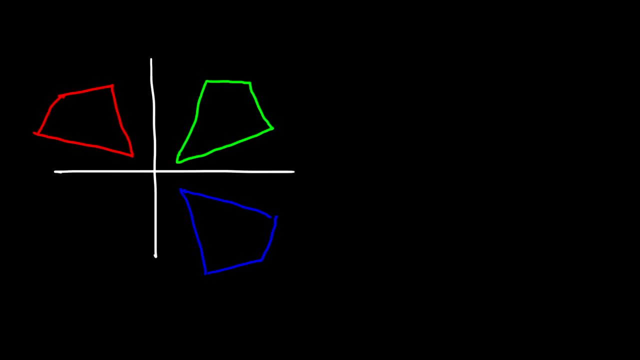 That's what I meant to say. So if we focus on a point, the x-value in quadrant 2 is negative, the y-value is positive. To reflect it about the origin, multiply the x and the y by negative 1.. So that point will be here. 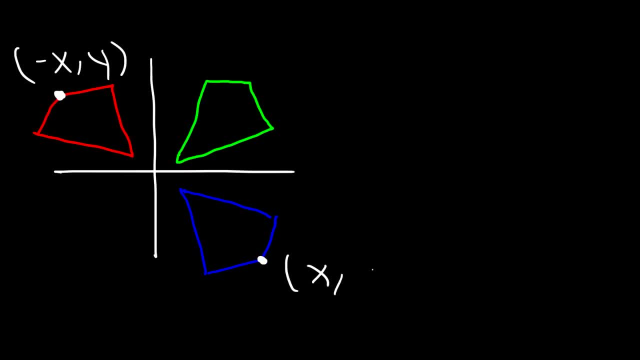 It's going to be positive x, negative y, So change the sign of both coordinates any time you need to reflect it. about the origin. Now let's work on some examples. So I want you to reflect this image about the x-axis. Let's call this point A, point B, point C. 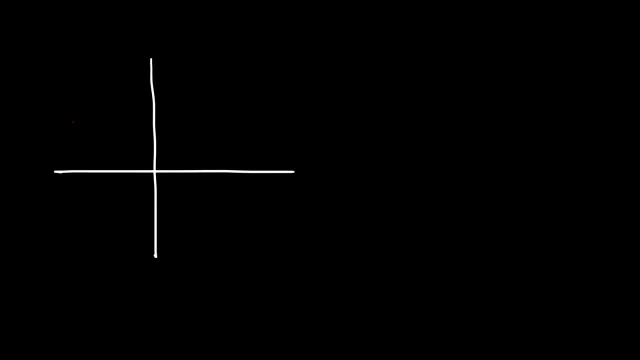 Let's say, if we have a figure that looks like this and it's in quadrant 2, draw a rough sketch of the image after reflection about the origin. So it's going to move from quadrant 2 to quadrant 4.. So if we reflect it about the y-axis first, it's going to look something like that: 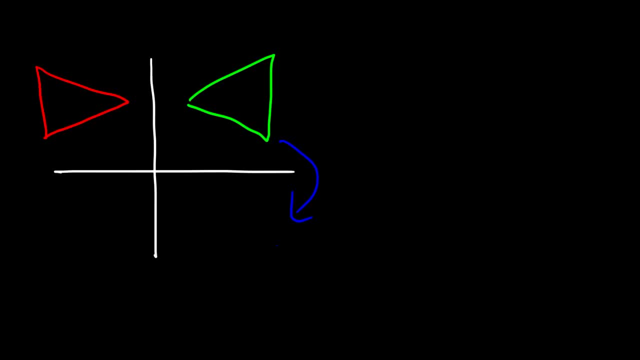 And then, if we reflect it over the x-axis, it's going to look like this. So, basically, the blue image is a reflection of the red image about the origin. Now let me change the structure. Let's say, if we have a shape, an unusually looking shape like this, let me make sure. 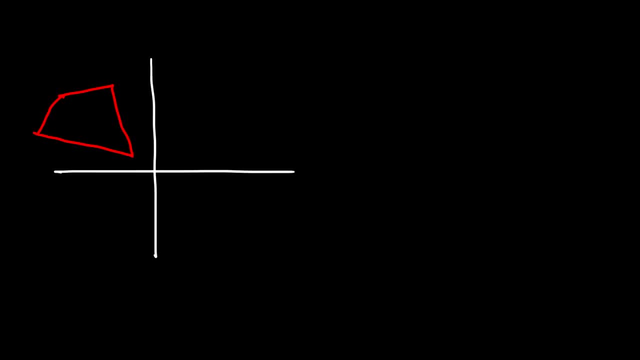 that one side is smaller relative to the other side. Reflect that image about the origin. So let's reflect it about the y-axis first. Okay, It's going to look something like that. And then, if we reflect it about the x-axis, it's going to look something like this: 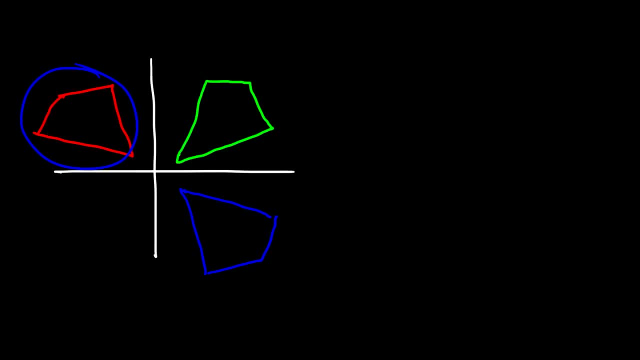 So this: the red one is a reflection of the blue one about the origin, or the blue one is a reflection of the red one about the origin. That's what I meant to say. So if we focus on a point, The x-value in quadrant two is negative, the y-value is positive. 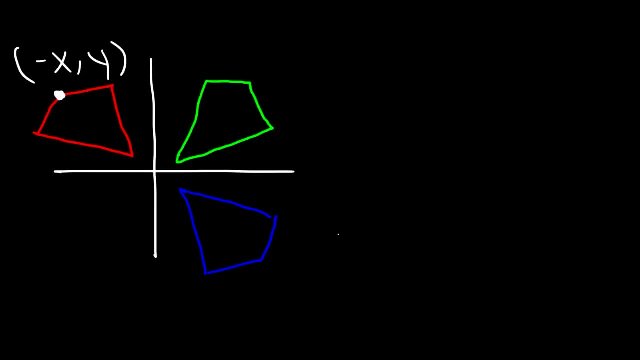 To reflect it about the origin, multiply the x and the y by negative one, So that point will be here. It's going to be positive x, negative y, So change the sign of both coordinates any time you need to reflect it about the origin. 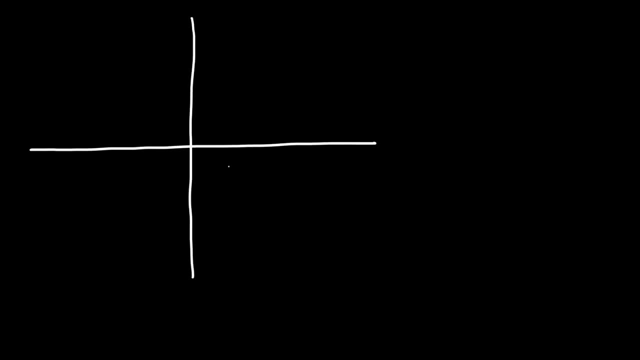 Now let's work on some examples. Okay, In this example, we're going to rotate this so that we see just the very question that 's left. Now the question is: how am I going to possibly tell these equations about? you know any? 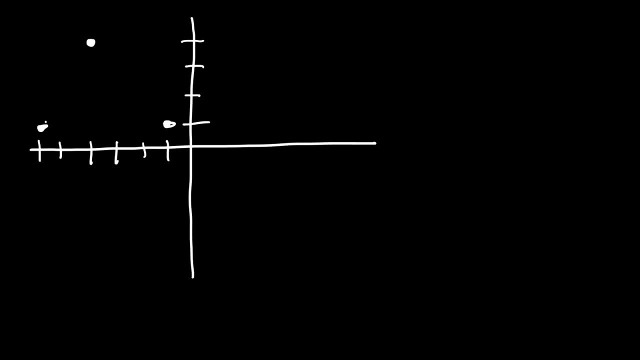 function that they do. Similarly, I can pick my argument with a negative. And what would happen now? Now, I would usually say, well, We'll do this. Number two is going to change The x-axis out the top here. Let's call this point A, point B, point C. 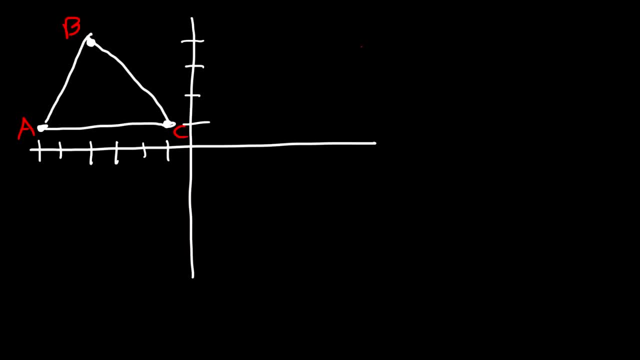 So go ahead and reflect it about the x-axis. So point A has the coordinates, Point B is located at And point C that's located at Now. in order to reflect it about the x-axis, we need to multiply the y-coordinates by negative. 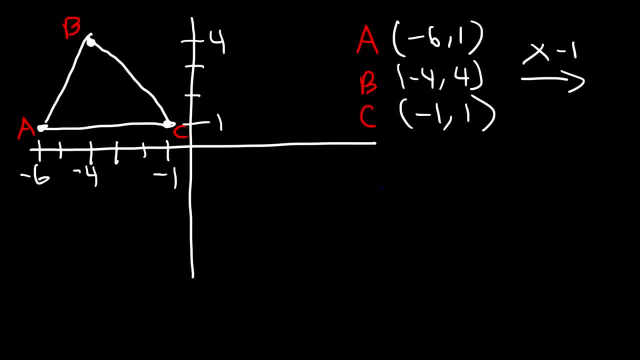 one. Okay, So therefore the new points for A, B and C are going to be So. all of the x-values will stay the same, Just change the y-values. So one is going to change to negative, one. Positive four will change to negative four. 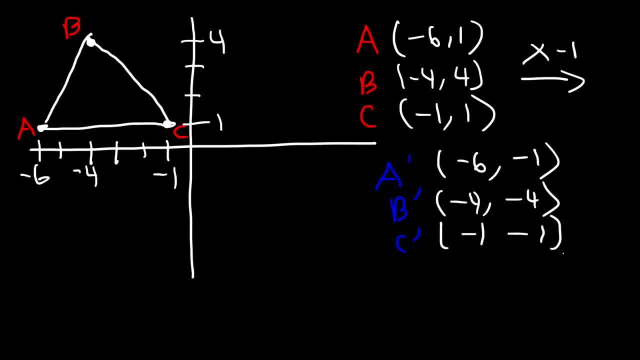 And this value will also change to negative one. So now we can plot the new figure. So let's say: Okay, Here's negative one. So the first point is at, which is here, The next one is at, and then 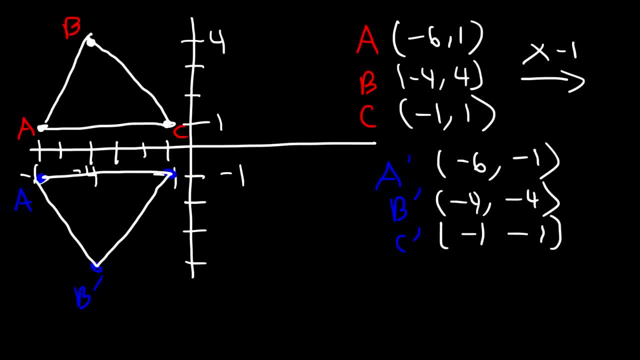 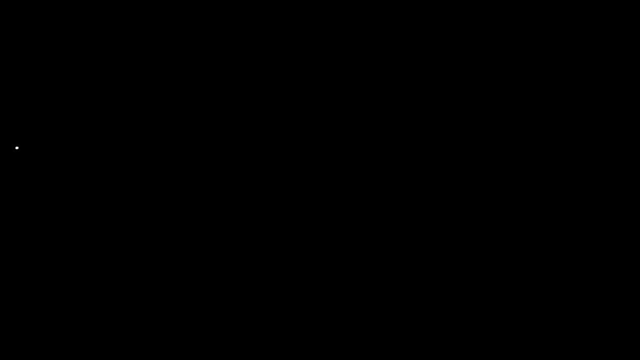 So this is going to be A, this is B and this is C. As you can see, it's a reflection. Okay, As you can see, it's a reflection about the x-axis, It's a mirror image about the x-axis. 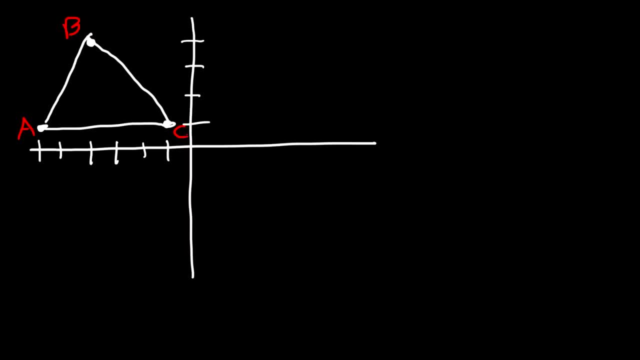 So go ahead and reflect it about the origin And reflect it about the x-axis. So point A has the coordinates, Point B is located at And point C that's located at Now in order to reflect it about the x-axis. 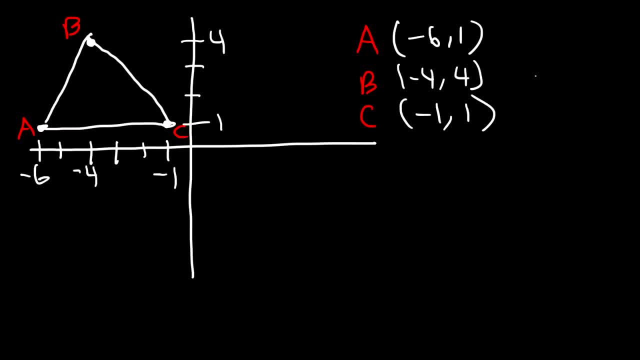 we need to multiply the y-coordinates by negative 1.. So therefore, the new points for A, B and C are going to be So: all of the x-values will stay the same, Just change the y-values. So 1 is going to change to negative 1.. 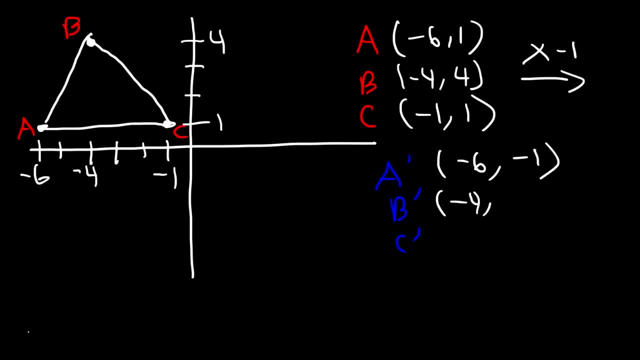 Positive 4 will change to negative 4.. And this value will also change to negative 1.. So now we can plot the new figure. So let's say, Here's negative 1.. So the first point is at, which is here: 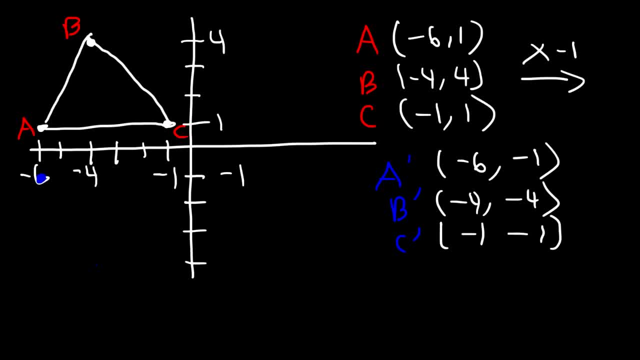 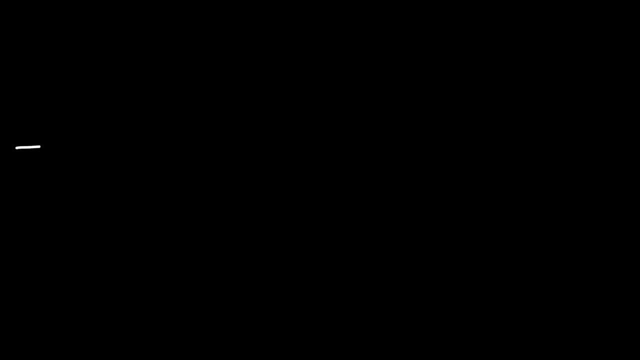 The next one is at and then. So this is going to be A, This is B And this is C. As you can see, it's a reflection about the x-axis, It's a mirror image about the x-axis. Now let's work on another example. 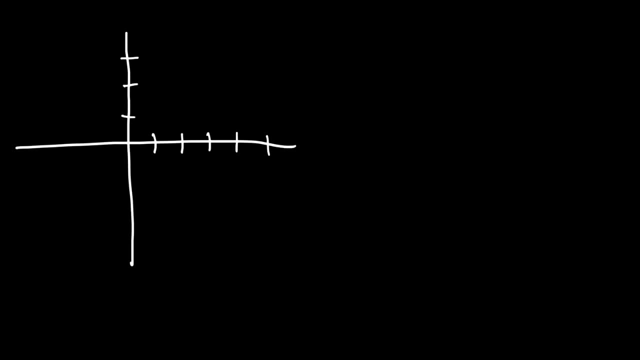 Go ahead and reflect this image about the y-axis. Let's say this is point A, B, C, D. So feel free to pause the video and work on that example. So let's find the coordinates of each point. So point A is located at: 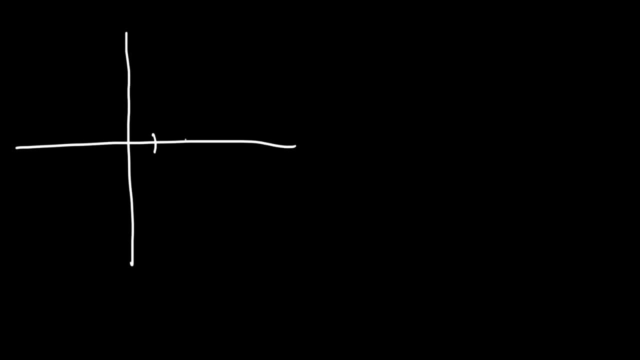 Now let's work on another example. Okay, Okay, Okay, Okay, Okay. Let's go ahead and have another example. Let's go ahead and reflect this image about the y-axis. Go ahead and reflect the image. Let's say: this is point A, B, C, D. 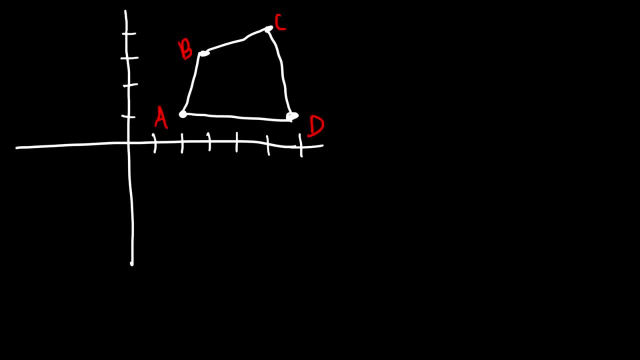 So feel free to pause the video and work on that example. Let's say: this is point A, B, C, D. So let's find the coordinates of each point. So let's find the coordinates of each point. So point A is located at, point B is located at. actually, that's not 2, that's. 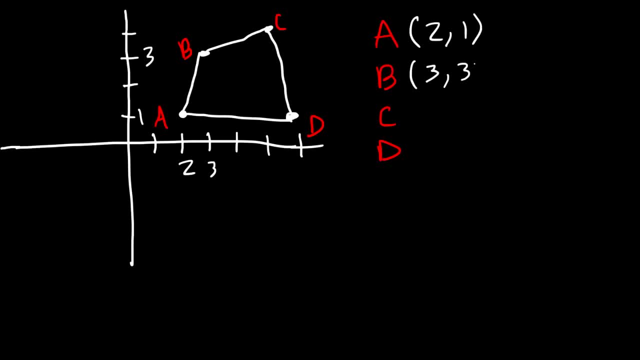 a y-value of 3,, so it's located at and C is located at and D is located at. So to reflect it about the x-axis- I mean not the x-axis, but rather the y-axis- we need to multiply the x-values by negative 1.. 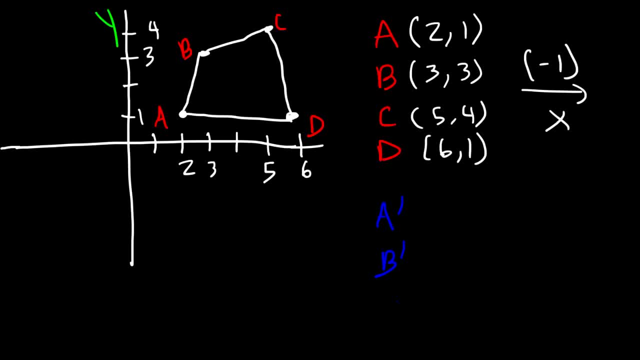 So now let's find the new coordinates. So instead of positive 2, it's going to change to negative 2.. The y-value will remain the same, So this is going to become negative 3, and then, instead of 5,, 4, it's going to be negative. 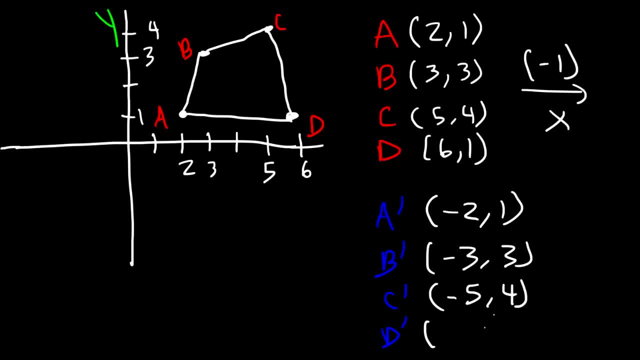 5, positive, 4, and D is going to change from 6, 1 to negative, 6, positive, 1.. So A is now located at, which is here, B is located at and C is located at and D is located at. 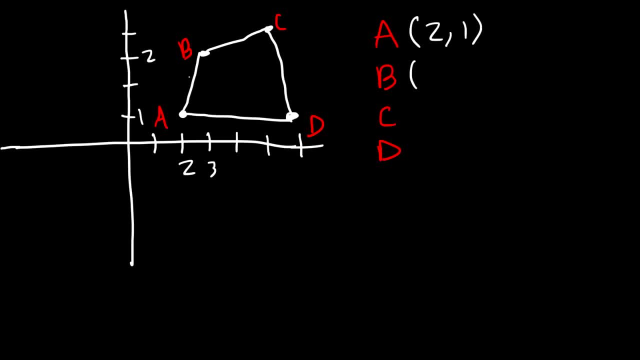 Point B is located at. Actually, that's not 2.. That's A y-value of 3. So it's located at, And C is located at, And D is located at. So to reflect it about the x-axis: 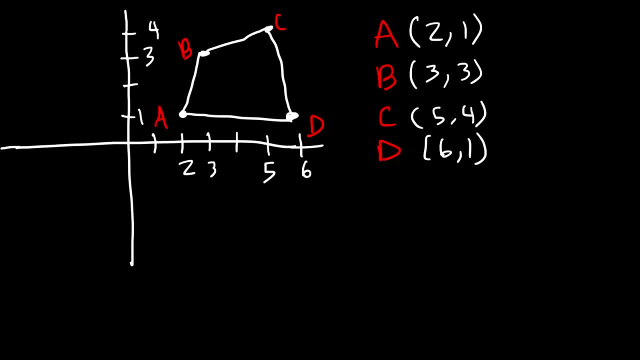 I mean not the x-axis, but rather the y-axis. we need to multiply the x-values by negative 1.. So now let's find the new coordinates. So instead of positive 2, it's going to change to negative 2.. 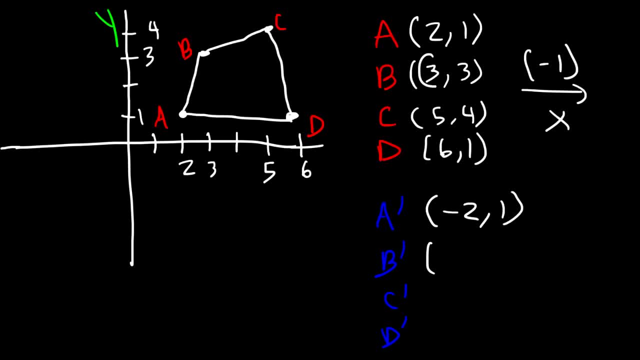 The y-value will remain the same. So this is going to become negative 3.. And then, instead of 5,, 4, it's going to be negative 5, positive, 4.. And D is going to change from 6, 1. 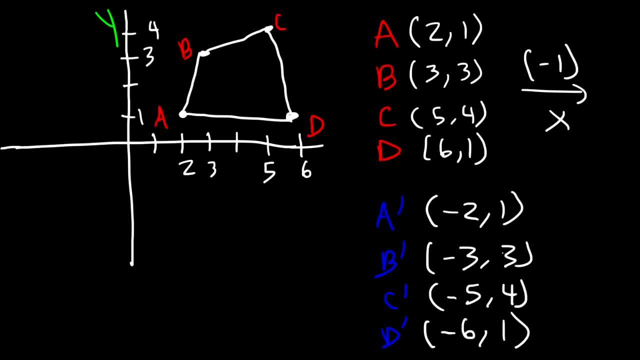 to negative 6, positive 1.. So A is now located at, which is here, B is located at and C is located at, And D is located at. So that's the reflected image over the y-axis. So all you need to do is multiply all coordinates. 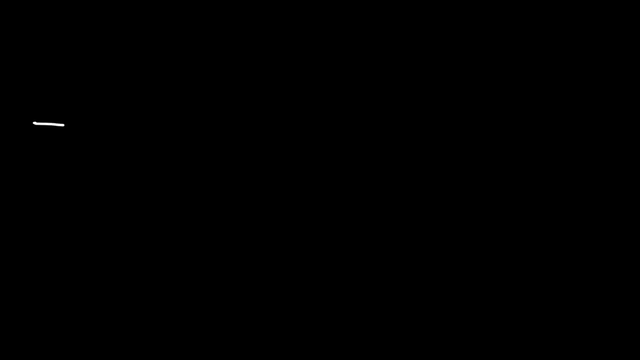 all x-coordinates by negative 1. Try this example. Reflect this image. about the origin: So let's call this point A, B and C. So take a minute, pause the video and reflect it. about the origin: So let's find the coordinates. 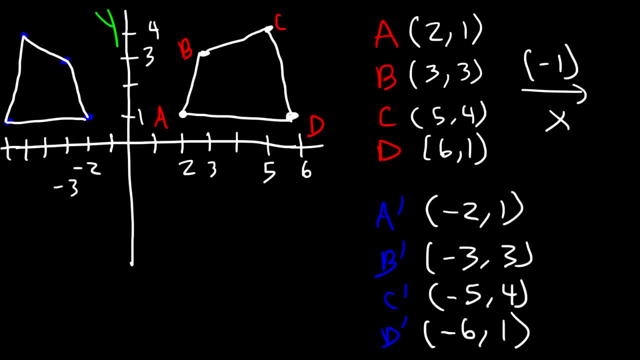 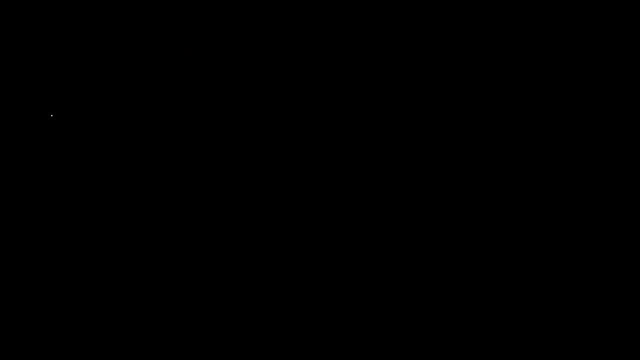 So that's the reflected image over the y-axis. So all you need to do is multiply all coordinates, All x-coordinates, by negative 1. Try this example. Reflect this image about the origin. So let's call this point A, B and C. 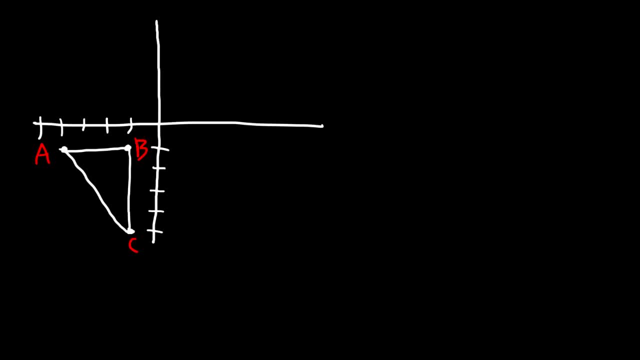 So take a minute, pause the video and reflect it about the origin. So let's find the coordinates of points A, B and C. A is located at. B is located at. B is located at. C is located at. 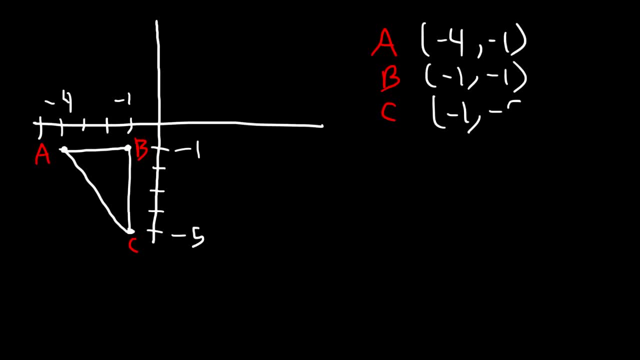 So now let's find the new coordinates. Any time you want to reflect it about the origin, multiply the x and the y coordinates by negative 1.. So A is going to change from negative 4, negative 1 to positive 4.. 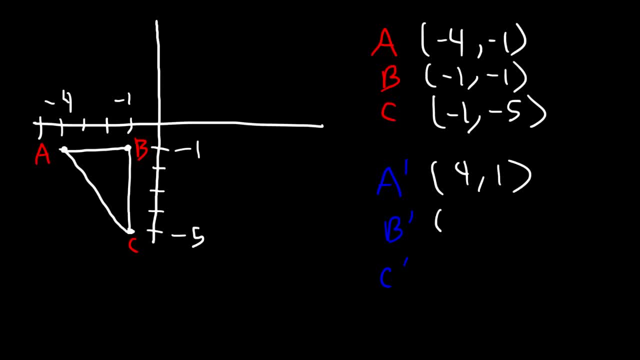 B is going to change from negative 4, negative 1 to positive 4.. So A is going to change from negative 4, negative 1 to positive 4.. B is going to change from negative 4, positive 1 to positive 1.. 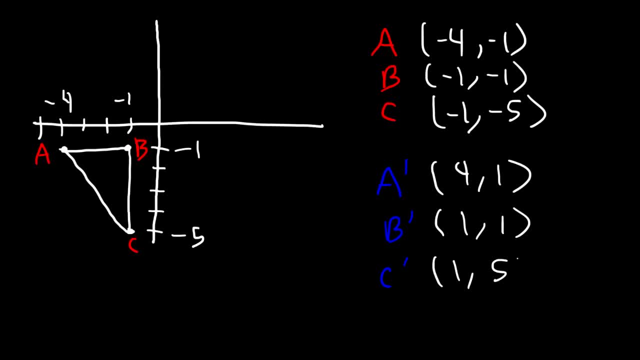 B is now going to be, C is going to be. So now let's go ahead and plot it. So A is at, B is at, C is at. So this is the new point for A, this is B, and that's the new point for C. 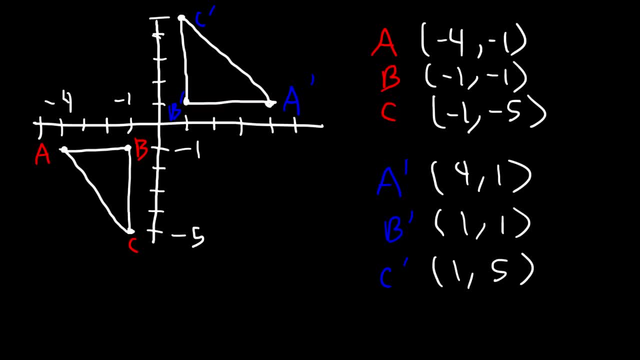 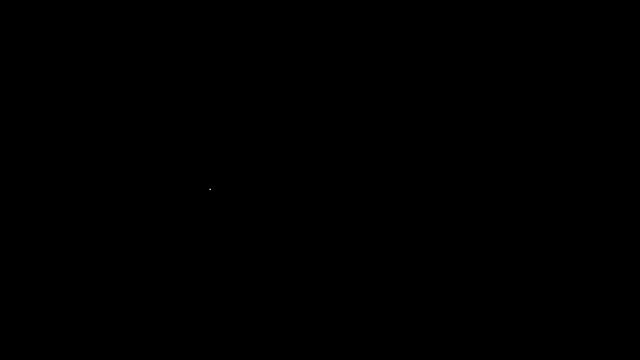 So that's how you can reflect an image over the origin if you have all the coordinates of the original figure. Now the last thing that we need to talk about are rotations. So let's say, if we have a triangle in Quadrant 1 and we wish to rotate it clockwise by 90, 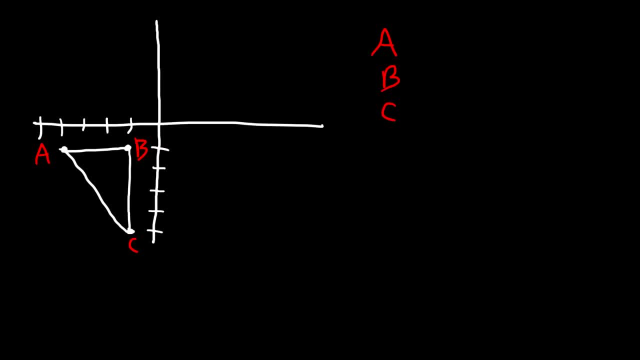 of points A, B and C. A is located at, B is located at and C is located at an x-value of but a y-value of. So now let's find the new coordinates Any time you want to reflect it about the origin. 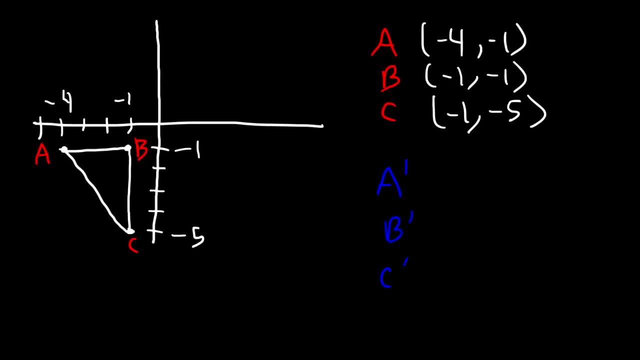 multiply the x and the y-coordinates by negative 1.. So A is going to change from to: B is now going to be, C is going to be. So now let's go ahead and plot it. So A is at. 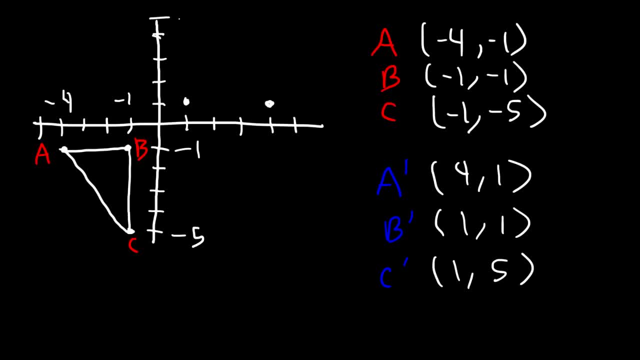 B is at, C is at. So this is the new point for A, this is B and that's the new point for C. So that's how you can reflect an image over the origin if you have all the coordinates of the original figure. 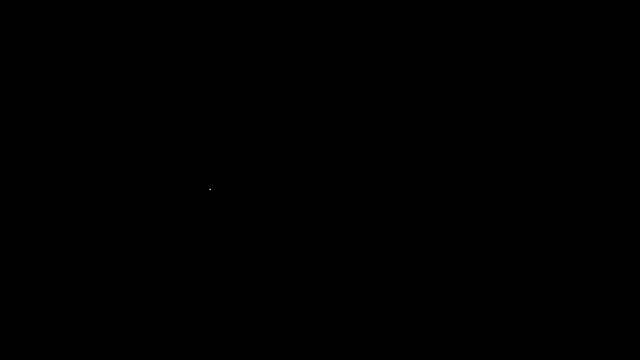 Now, the last thing that we need to talk about are rotations. So let's say, if we have a triangle in quadrant 1, and we wish to rotate it clockwise by 90 degrees, So if it's in quadrant 1, and we rotate it clockwise, 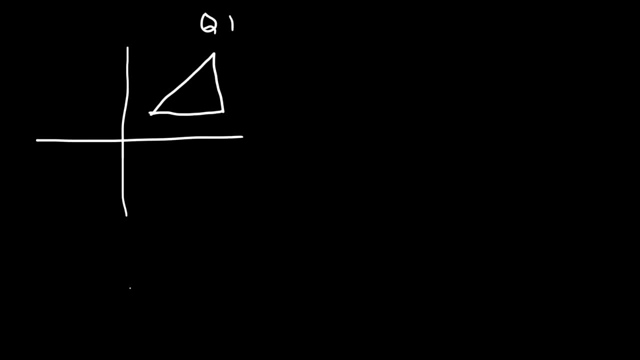 it's going to be in quadrant 4. And it's going to look like this. So let's say, if this is A, B and C, this point is now A, this is B and this is C, If we make it a right triangle. 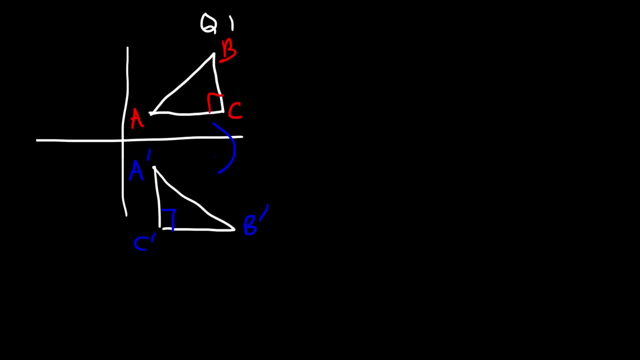 C is the hypotenuse of the right triangle. So that's rotated. so that's rotating the figure 90 degrees clockwise. Now what about rotating the figure 90 degrees counterclockwise? So let's start with the same original picture. 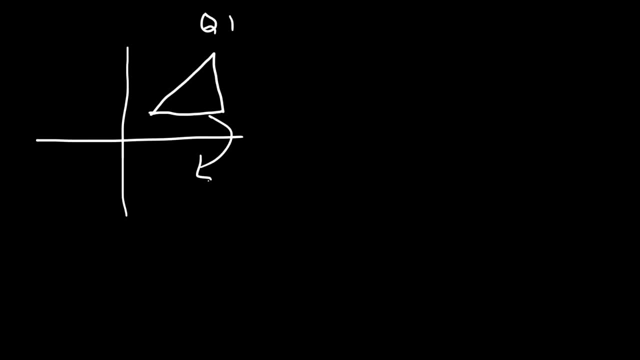 degrees. So if it's in Quadrant 1 and we rotate it clockwise, it's going to be in Quadrant 4 and it's going to look like this. So let's say, if this is A, B and C, This point is now A. 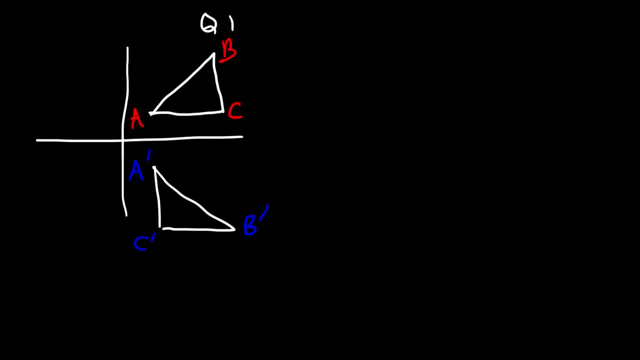 This point is now B, This is B and this is C. If we make it a right triangle, C is the hypotenuse of the right triangle. So that's rotating a figure 90 degrees clockwise. Now, what about rotating a figure 90 degrees counterclockwise? 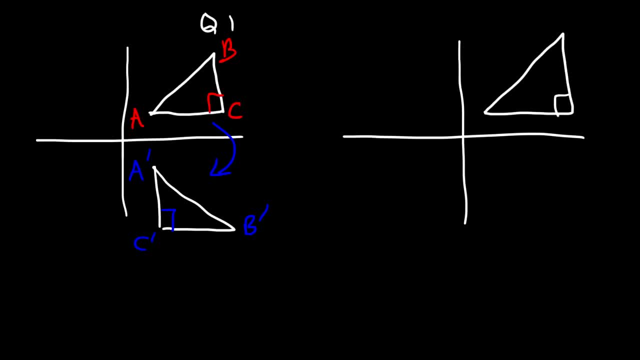 So let's start with the same original picture. If we rotate it counterclockwise, it's going to move from Quadrant 1 to Quadrant 2.. So if we rotate it counterclockwise, it's going to move from Quadrant 1 to Quadrant. 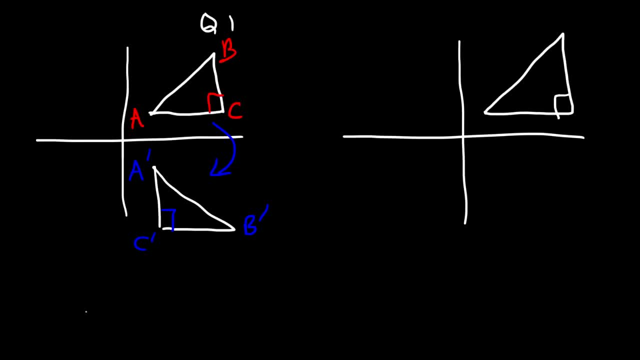 2. So if we rotate it counterclockwise, it's going to move from Quadrant 1 to Quadrant 2.. So, therefore, you're going to get a picture that looks like this: So using the same letters. this is now point A. 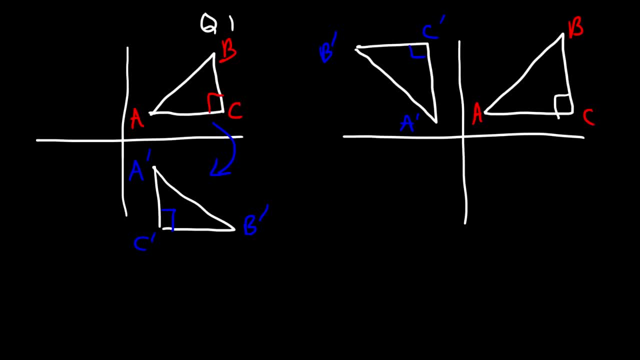 That's B And this is C. So that's the 90 degree rotation, counterclockwise, See. And the first example was in the direction of a clock. Now, what about rotating a figure by 180 degrees? The direction that you choose to take doesn't matter. 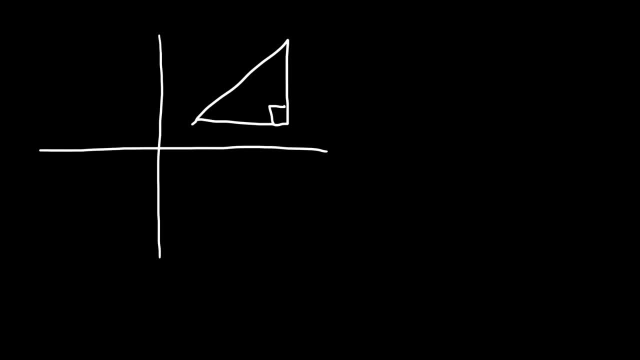 Right now we have a triangle in quadrant 1. And if we choose to rotate it by 180 degrees in a counterclockwise direction, it's going to move from quadrant 1 to quadrant 3.. If we rotate it in the clockwise direction, it's still going to end in quadrant 3.. 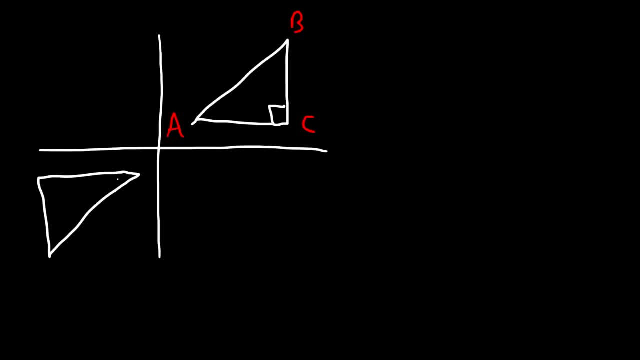 And you're going to get the same exact shape. So a rotation of 180 degrees has the same effect as reflecting a graph across the origin. So this is C, this is A and this is point B. Now, if you need to rotate, 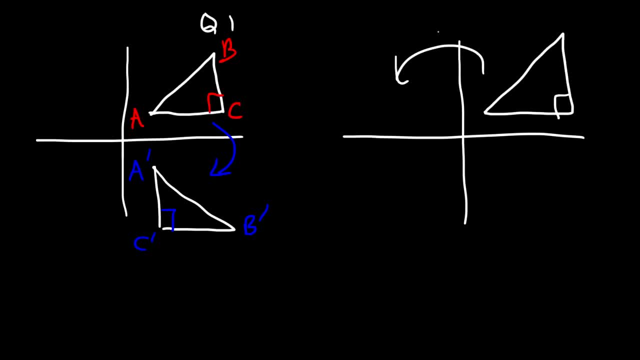 If we rotate it counterclockwise, it's going to move from quadrant 1 to quadrant 2.. So, therefore, you're going to get a picture that looks like this. So, using the same letters, this is now point A, that's B. 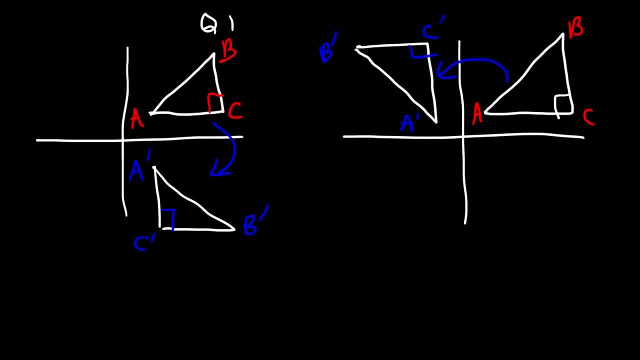 and this is C. So that's a 90 degree rotation, counterclockwise, And the first example was in the direction of a clock. Now what about rotating a figure by 180 degrees? The direction that you choose to take doesn't matter. 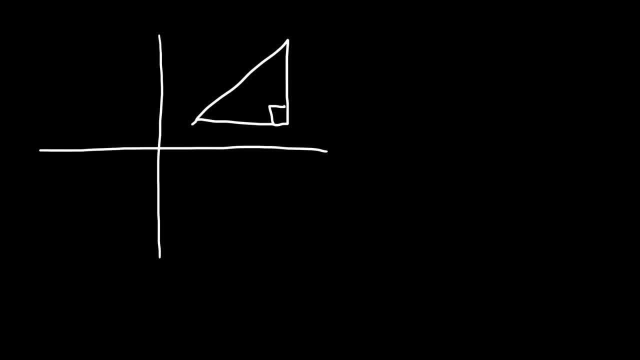 Right now we have a triangle in quadrant 1. And if we choose to rotate it by 180 degrees in the counterclockwise direction, it's going to move from quadrant 1 to quadrant 3.. If we rotate it in the clockwise direction, 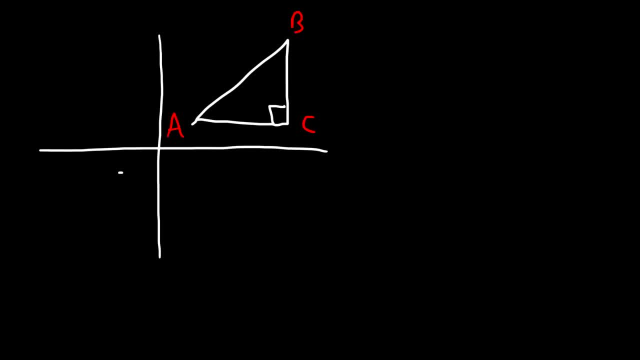 it's still going to end in quadrant 3. And you're going to get the same exact shape. So a rotation of 180 degrees has the same effect as reflecting a graph across the origin. So this is C, this is A and this is point B. 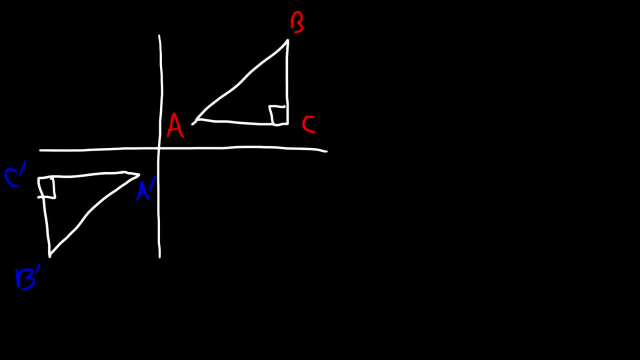 Now, if you need to rotate the graph by 180, all you need to do is change the coordinates. You need to multiply each coordinate by negative 1.. So if you have the point, it's going to change to. If you need to rotate it by, 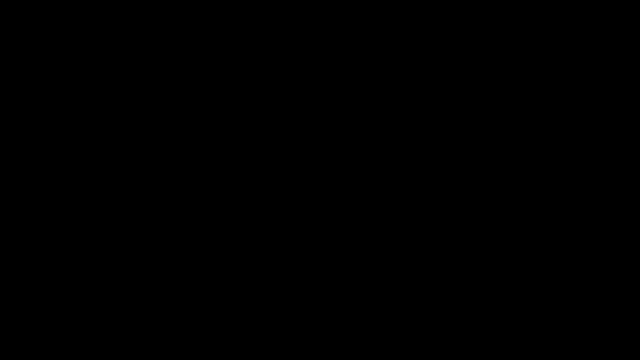 180 degrees. Now let's say, if you want to rotate it 90 degrees clockwise, And let's say the original point is in quadrant 1. It's What you need to do, is you need to switch the coordinates of each point. 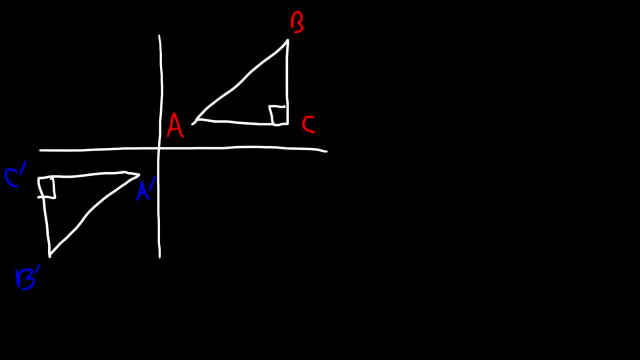 the graph by 180,. all you need to do is change the coordinates. You need to multiply each coordinate by negative 1. So if we have the point X, Y, it's going to change to negative X, negative Y. If you need to rotate it by 180 degrees. 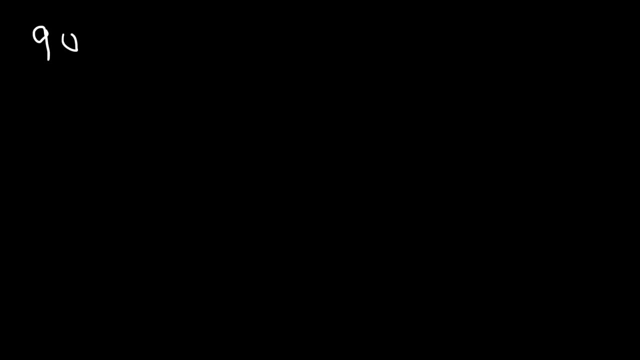 Now let's say, if you want to rotate it 90 degrees clockwise, And let's say the original point is in quadrant 1.. It's X- Y. What you need to do is you need to switch the coordinates of each point, So it's going to be Y- X. 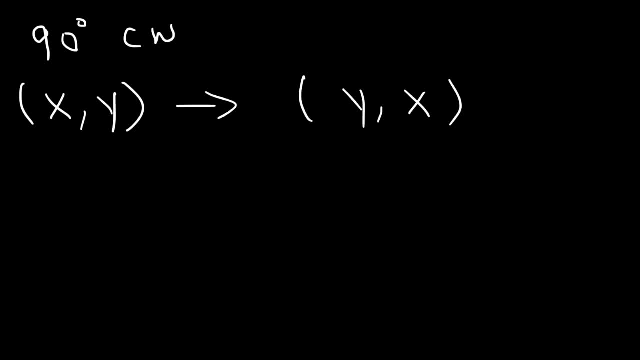 And then the new second coordinate. you need to multiply it by negative 1.. So this is the new second coordinate. Now, in the case of a rotation that's 90 degrees counterclockwise, you're going to switch the coordinates once again. 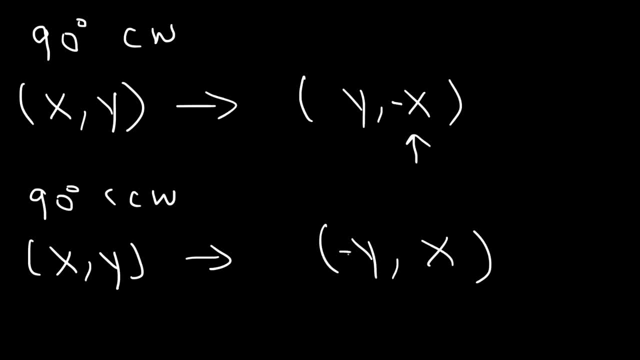 But this time you're going to multiply the first coordinate by negative 1.. Let's try an example. Go ahead and rotate this figure 90 degrees clockwise. So let's say this is point A, B and C. So let's begin by writing each point. 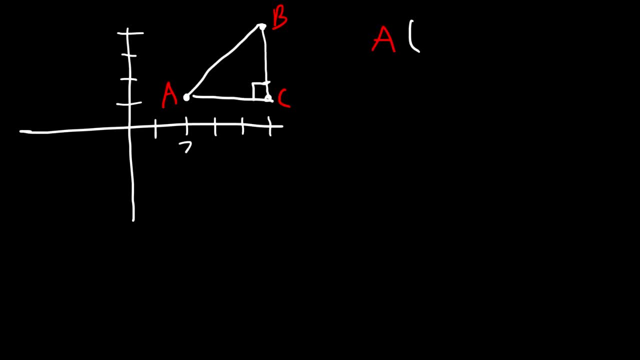 Point A is located at 2, 1.. Next we have point B, which is located at 5, 4.. And point C is located at 5, 1.. So to rotate it clockwise, what we need to do if we're going to rotate 90 degrees clockwise about the origin: 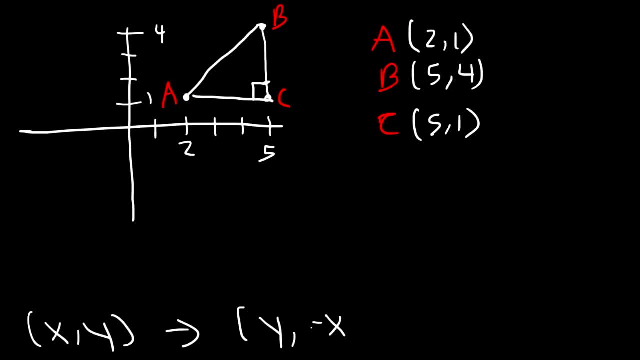 we need to switch the coordinates and then multiply the second coordinate by negative 1.. So let's find the new values. So first we're going to switch 2, 1, and it's going to become 1, 2.. 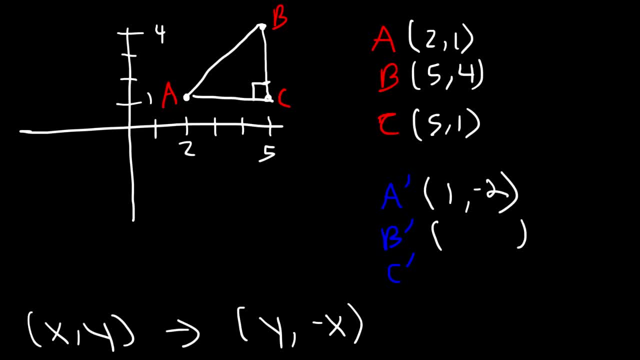 But the second coordinate we're going to make it negative. For B, instead of 5, 4, it's going to be 4, 5, but negative 5.. And for C it's going to be 1, negative 5.. 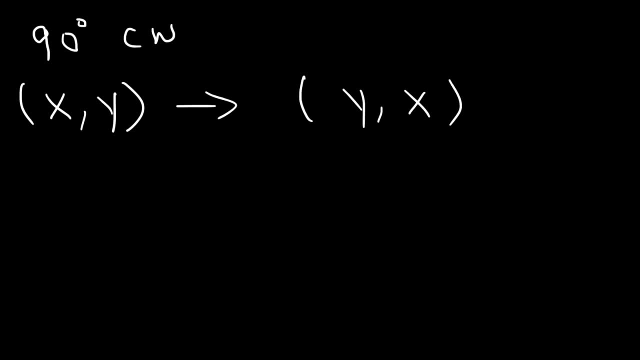 So it's going to be. And then the new second coordinate. you need to multiply it by negative 1.. So this is the new second coordinate. Now, in the case of a rotation that's 90 degrees counterclockwise, you're going to switch the coordinates once again. 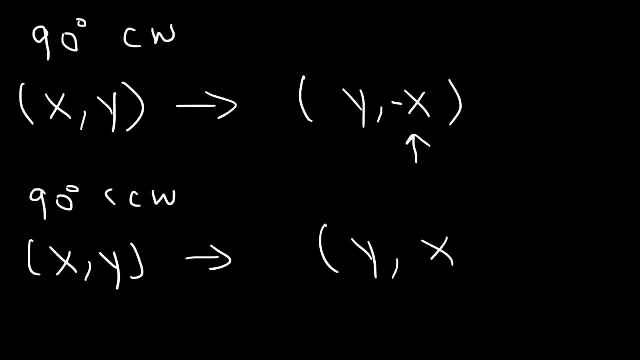 But this time you're going to multiply the first coordinate by negative 1.. Let's try an example. Go ahead and rotate this figure 90 degrees clockwise. So let's say this is point A, B and C. So let's begin by writing each point. 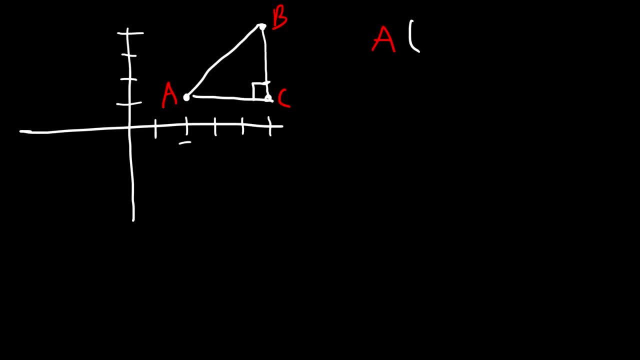 Point A is located at. Next we have point B, which is located at And point C is located at. So to rotate it clockwise, what we need to do if we're going to rotate 90 degrees clockwise about the origin, we need to switch the coordinates. 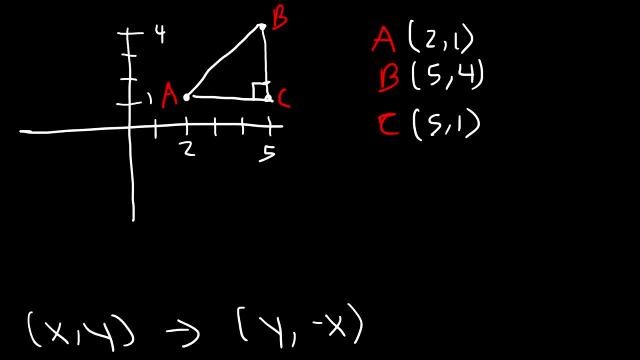 and then multiply the second coordinate by negative 1.. So let's find the new values. So first we're going to switch to 1, and it's going to become, But the second coordinate, we're going to make it negative. 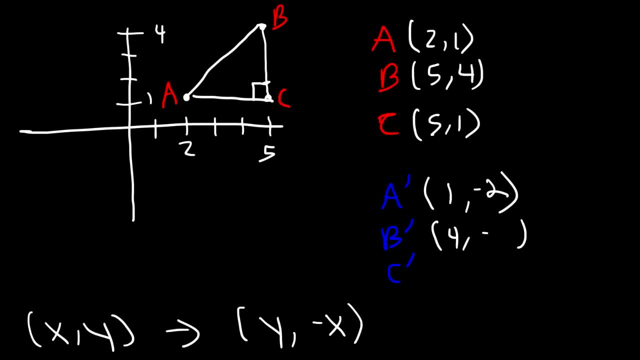 For B instead of it's going to be but negative 5. And for C it's going to be. So now let's plot the new points that we have. So the first one is at: which is right here? 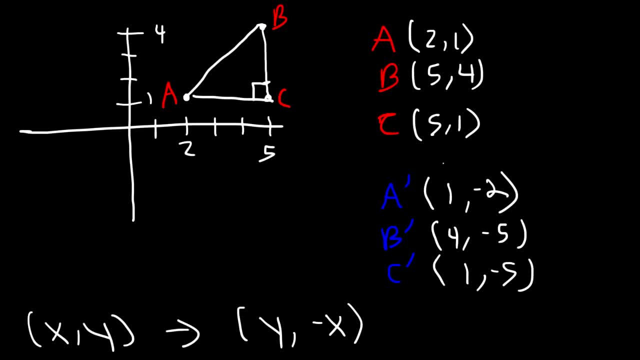 So now let's plot the new points that we have. So the first one is at 1, negative 2, which is right here. The next one is at 4, negative 5.. And the next point is at 1, negative 5.. 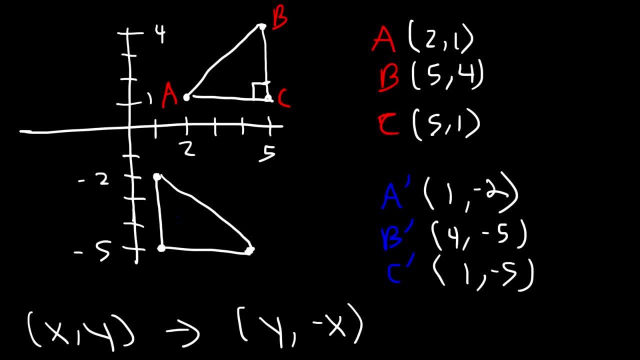 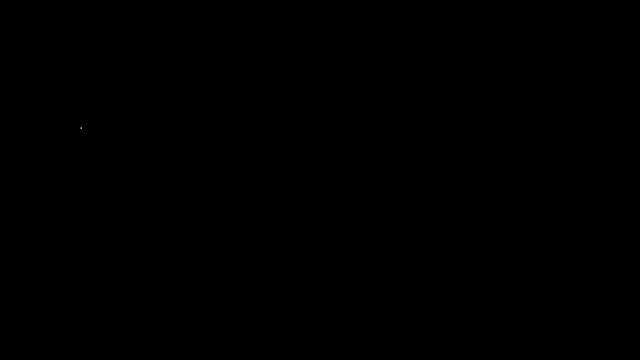 So this is the image that we now have. so this is a, B is that four negative five, and this is C. so, as you can see, we've rotated it 90 degrees clockwise. let's try another example. so rotate this figure 90 degrees counterclockwise. so go ahead and take a. 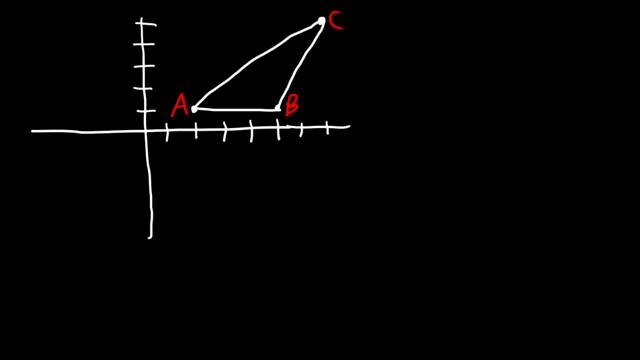 minute and work on this problem. so first let's write the three points that we have. point a is located at 2: 1, point B is located at 5 comma 1 and C is located at 7 comma 5. now, if you want to rotate it 90 degrees counterclockwise, the first thing you 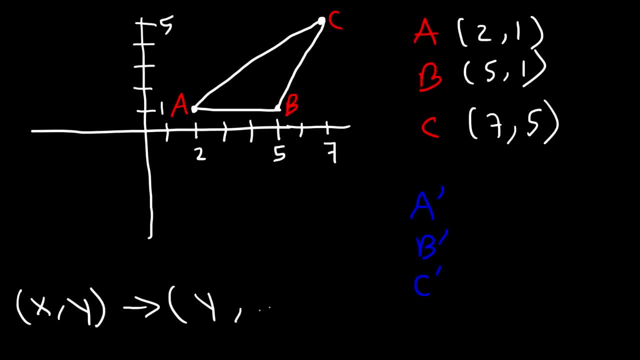 need to do is switch X and Y and then you're going to multiply the first coordinate by negative 1. so we're going to switch the point 2, 1 and it's going to become 1 comma 2, and then multiply the first coordinate by negative 1. we're going to 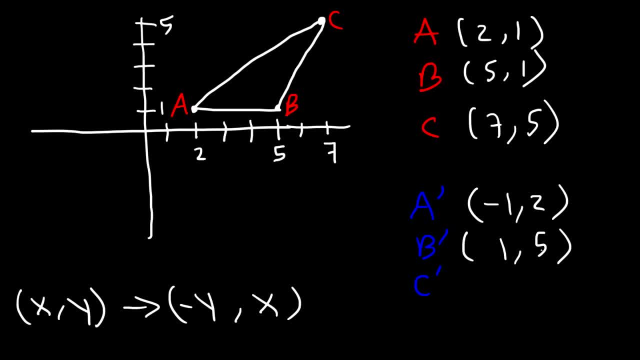 switch 5- 1 into 1, 5 and then add a negative sign to the first coordinate and 7: 5 is going to become 5: 7. but we're going to multiply the first corner by negative 1. so all of these points, they're located in: 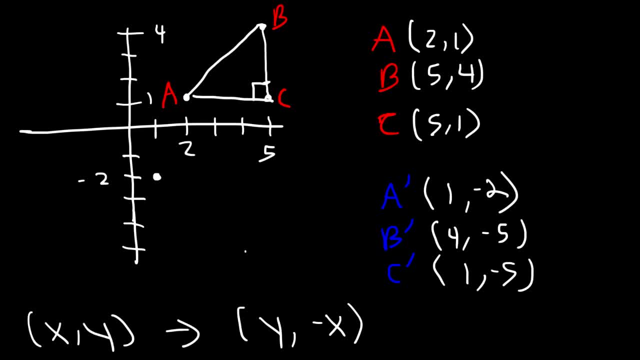 The next one is at negative 5. And the next point's at negative 5.. So this is the image that we now have. So this is A, B is at and this is C. So as you can see, 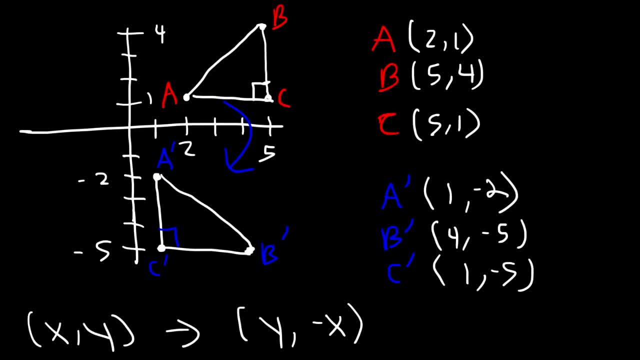 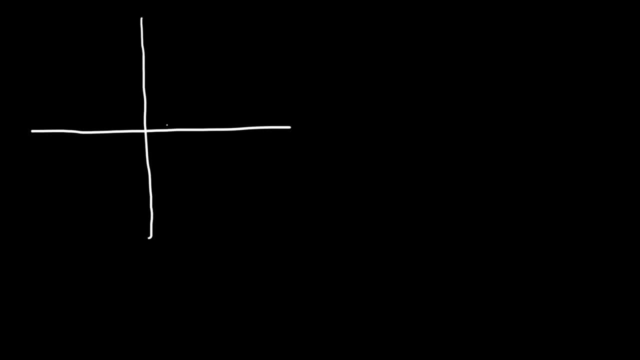 we've rotated it 90 degrees clockwise. Let's try another example. So rotate this figure 90 degrees counterclockwise. So go ahead and take a minute and work on this problem. So first let's write the three points that we have. 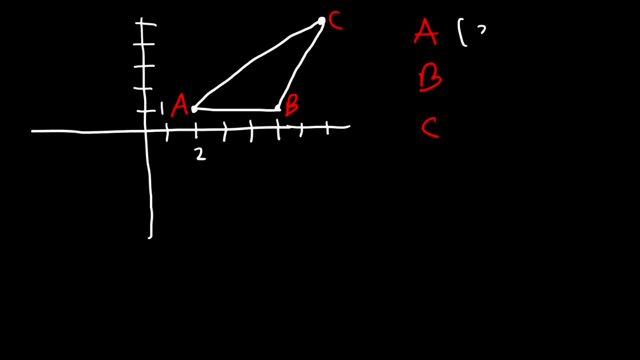 Point A is located at, Point B is located at And C is located at Now. if you want to rotate it 90 degrees counterclockwise, the first thing you need to do is switch X and Y, And then you're going to multiply the first coordinate. 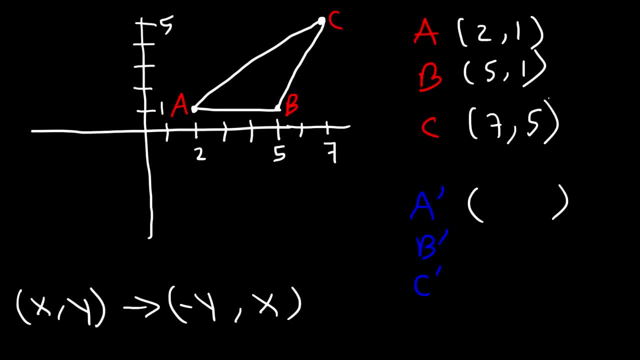 by. So we're going to switch the point to 1, and it's going to become, and then multiply the first coordinate by. We're going to switch into and then add a negative sign to the first coordinate And is going to become. 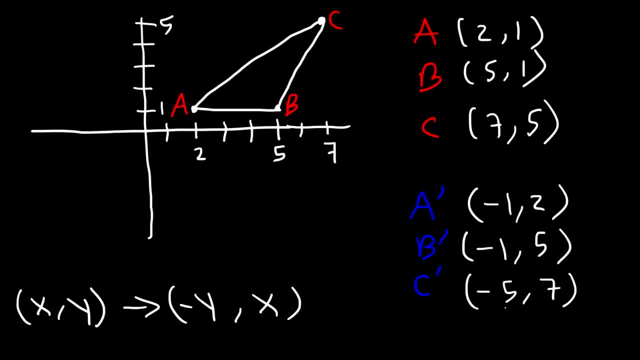 but we're going to multiply the first coordinate by So all of these points they're located in. So the first one is located at, which is here. The second point is: The third point is, which I'm running out of space. 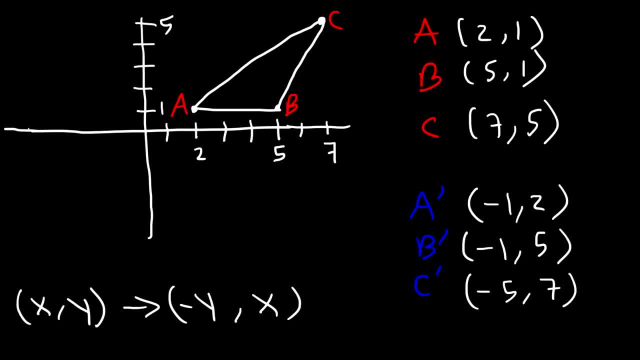 quadrant 2. so the first one is located at negative 1 comma 2, which is here. the second point is negative 1, 5. the third point is negative 5 comma 7, which i'm running out of space, so i'm So I'm just going to put it on top here somewhere. 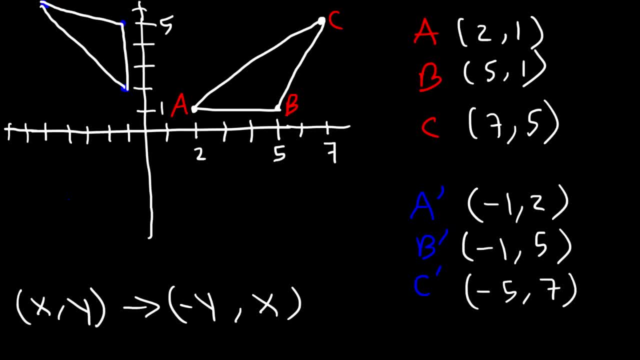 So that's a rough sketch of what the new graph should look like. So this is A, this is B and this is C. So it rotated 90 degrees in the counterclockwise direction. So we're going to look at one final example. 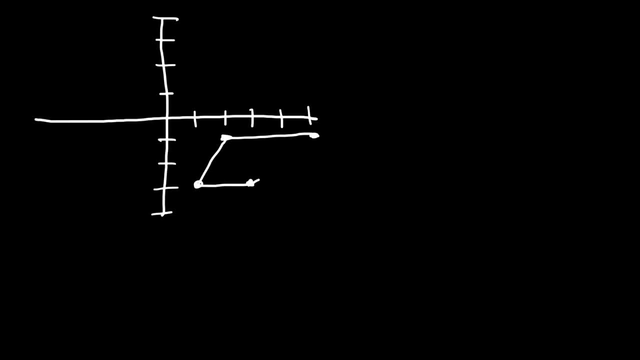 Go ahead and rotate this figure by 180 degrees clockwise. So let's call this A, B, C and D. So go ahead and work on this problem. So A is located at 2, negative 1. B is located at 5.. 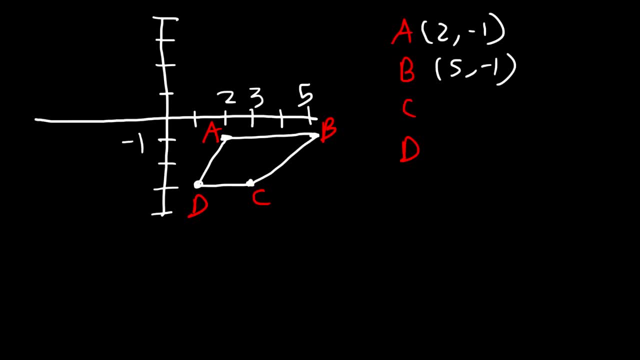 5, negative 1.. C is located at 3, negative 3.. And D is located at 1, negative 3.. Now, when rotating it about 180, regardless of the direction, all you need to do is multiply the points by negative 1.. 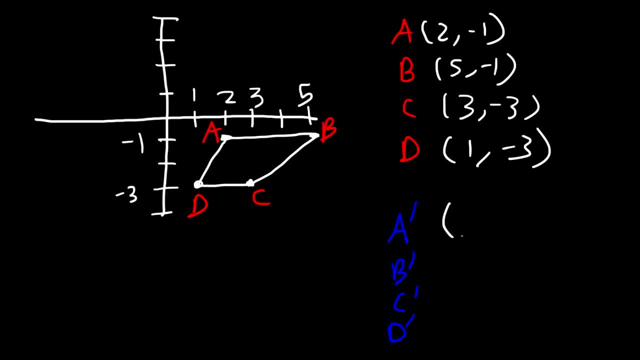 That's all you have to do. So A is going to change from 2, negative 1. To negative 2, positive 1.. B is going to become negative 5, 1.. C is going to change to negative 3, 3.. 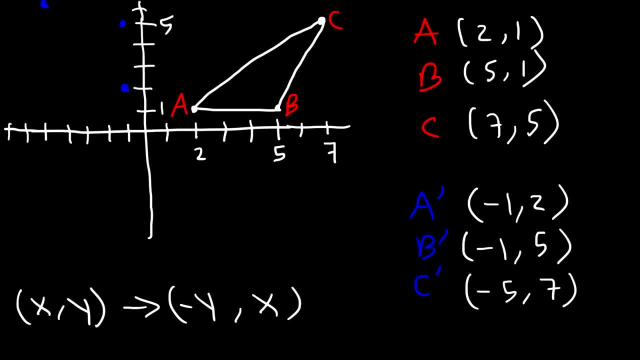 so I'm just going to put it on top here somewhere. So that's a rough sketch of what the new graph should look like. So this is A, this is B and this is C. So it rotated 90 degrees in the counterclockwise direction. 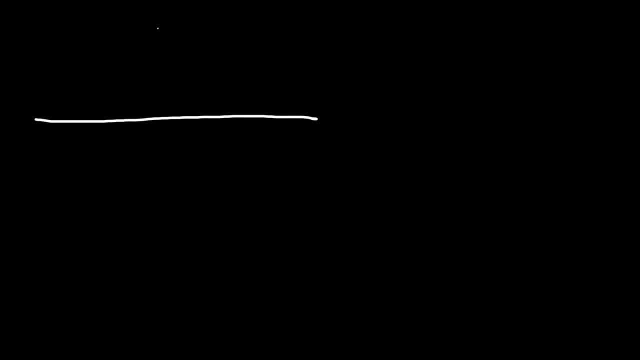 So we're going to look at one final example. Go ahead and rotate this figure by 180 degrees clockwise. So let's call this A, B, C and D. So go ahead and work on this problem. So A is located at. 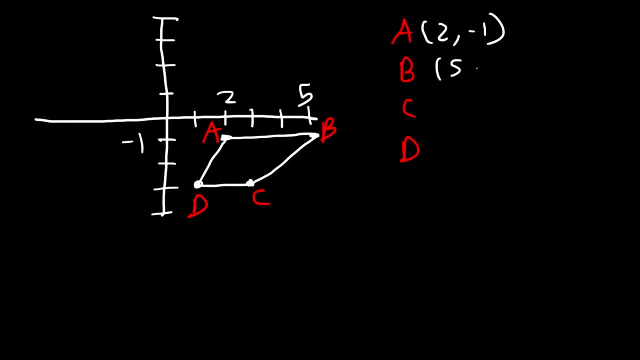 B is located at, C is located at And D is located at. Now, when rotating it about 180, regardless of the direction, all you need to do is multiply the points by. That's all you have to do. So A is going to change from to: 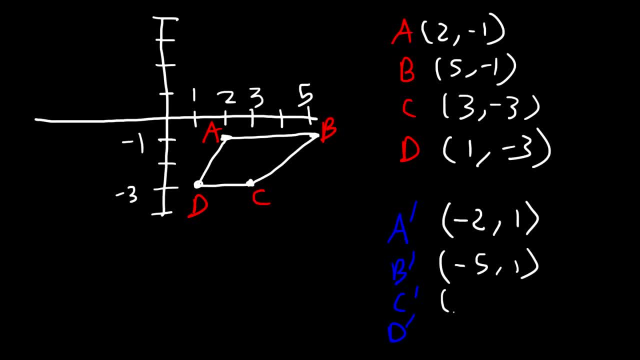 B is going to become, C is going to change to And D is going to be. So. the points will change to: Just multiply each coordinate by. So A is at And then B is at, So that's A. This is B. 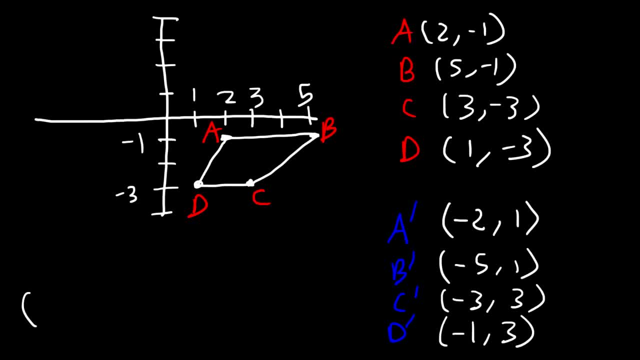 And D is going to be negative 1,, positive 3.. So the points will change to negative x, negative y. Just multiply each coordinate by negative 1.. So A is at negative 2, 1.. And then B is at negative 5, 1.. 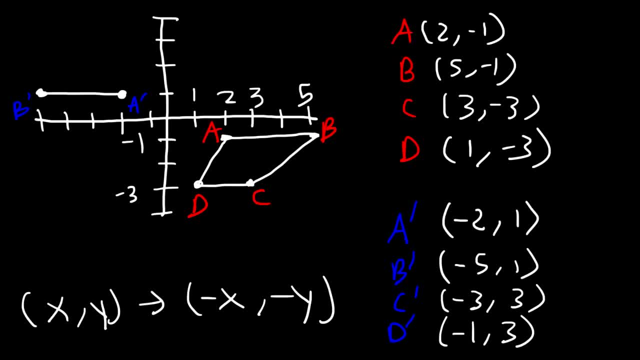 So that's A, This is B And then C is located at negative 3, 3.. And D is located at negative 1, 3.. And that's it. So if you take it one step at a time, you can easily plot the rotation or reflection. 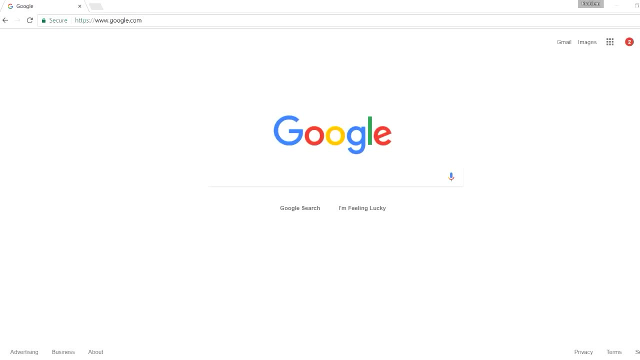 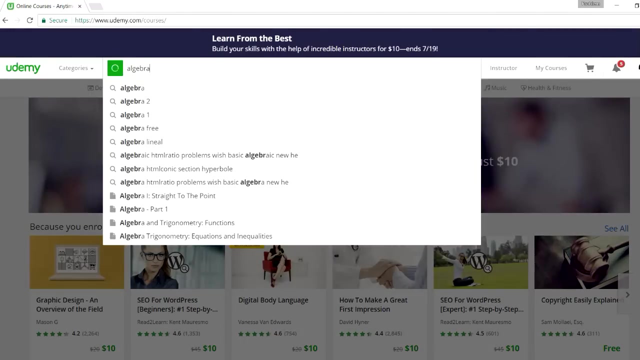 Now I want to show you one of my algebra courses that might be useful to you if you ever need it. So go to udemycom Now in the search box just type in algebra And it should come up. And it should come up. 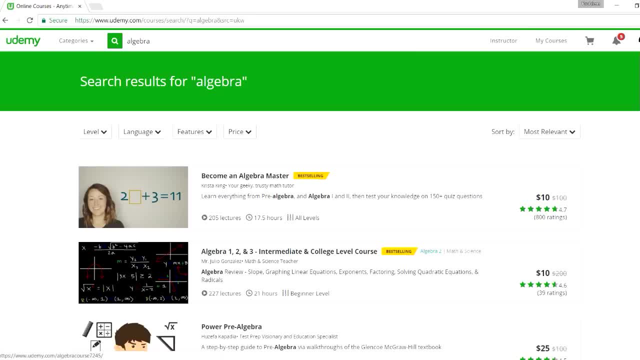 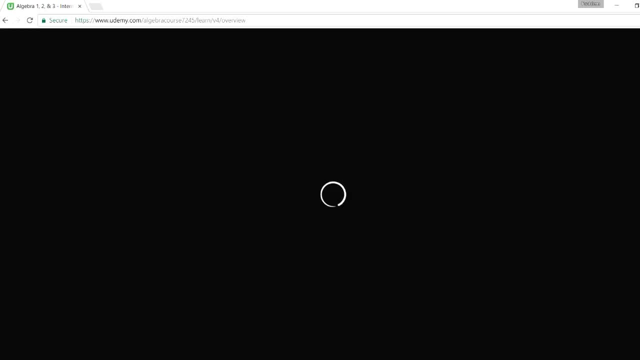 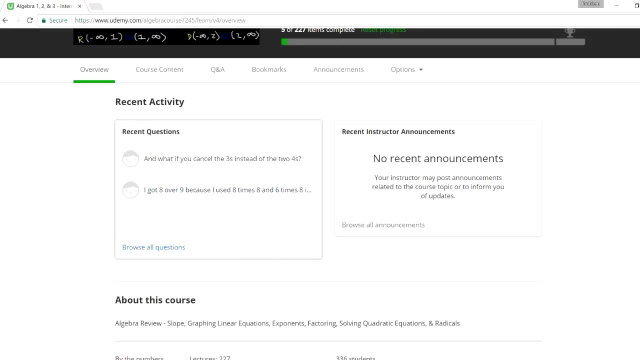 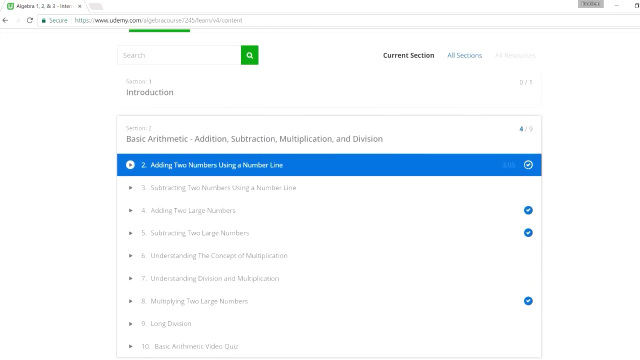 So it's the one with the image with the black background. So if you select that option and if you decide to go to course content, you can see what's in this particular course. So the first section, basic arithmetic. for those of you who want to focus on addition, 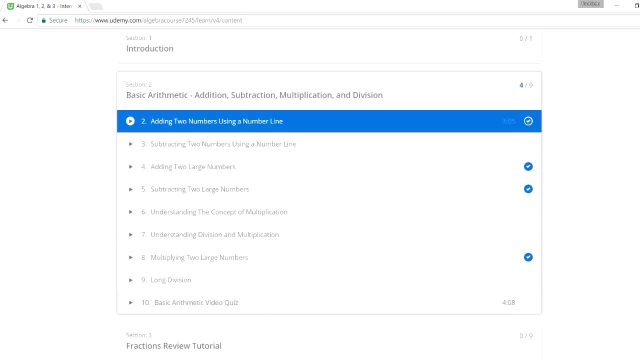 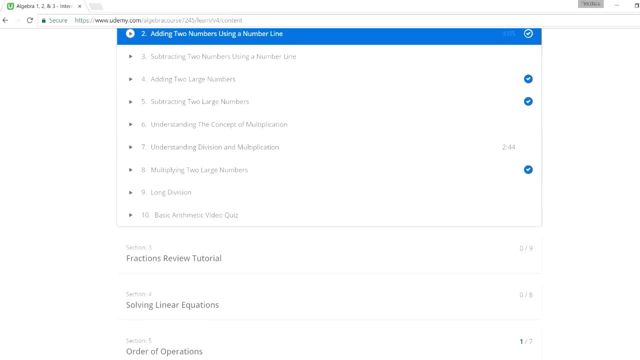 subtraction, multiplication and division And it has a video quiz at the end. It's a multiple choice video quiz. You can pause it, work on the problems and see the solutions. It covers long division, multiplying two large numbers and things like that. 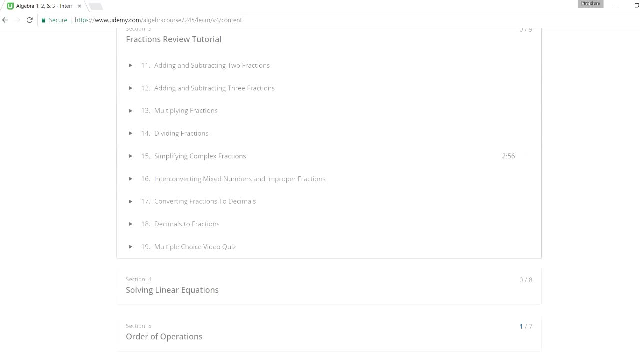 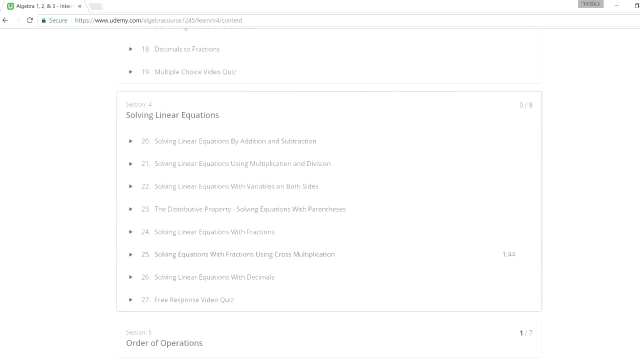 The next tutorial is on fractions: Adding, subtracting fractions, multiplying and dividing fractions, Converting fractions into decimals and so forth, So you can also take a look at that. Next, solving linear equations, which we covered, And just more examples if you need more help with that. 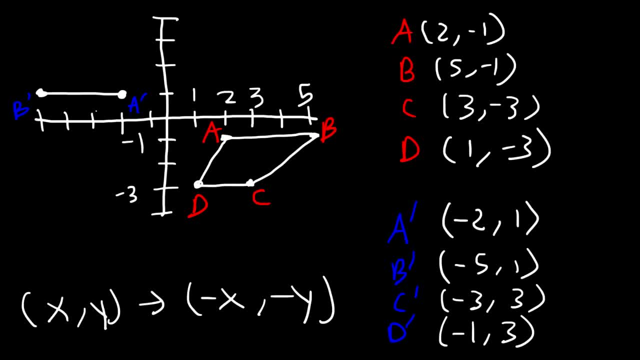 And then C is located at And D is located at Three, And that's it. So if you take it one step at a time, you can easily plot the rotation or reflection. Now I want to show you one of my algebra courses. 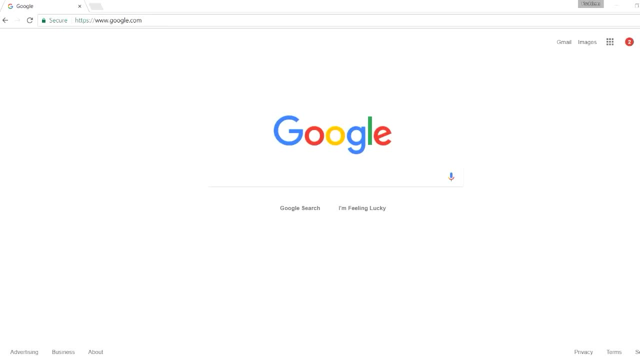 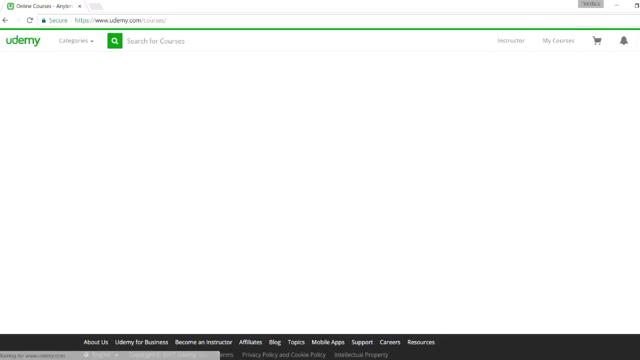 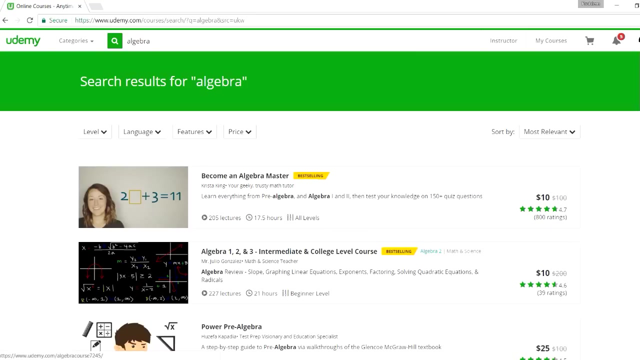 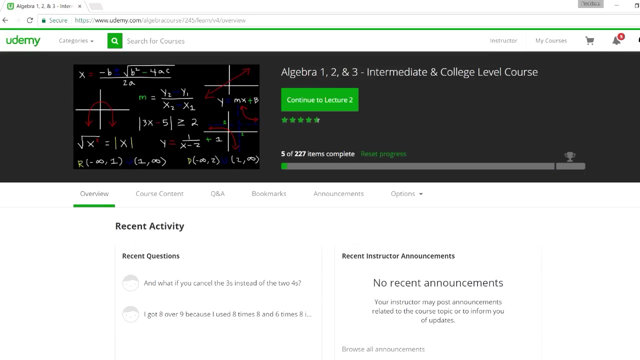 that might be useful to you if you ever need it. So go to udemycom Now in the search box just type in algebra And it should come up. So it's the one with the image with the black background. So if you select that option, 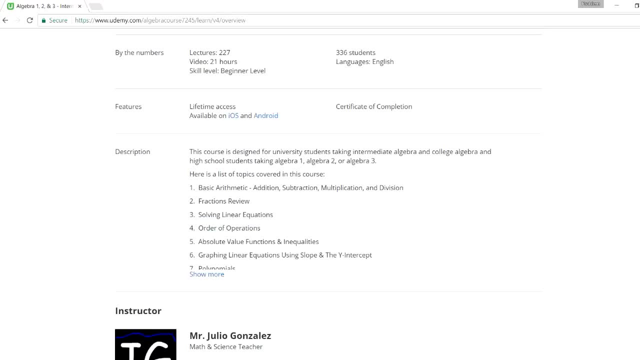 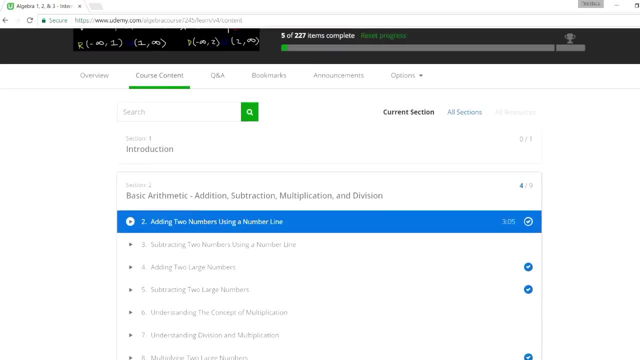 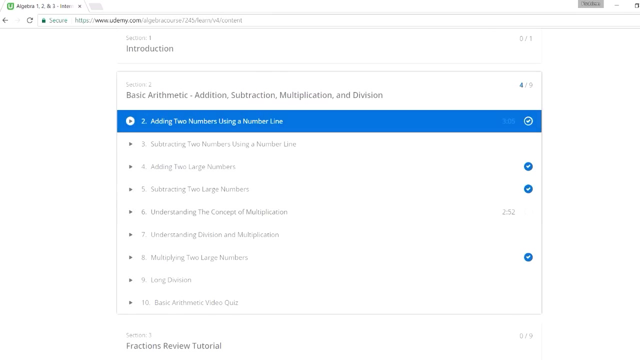 and if you decide to go to course content, you can see what's in this particular course. So the first section, basic arithmetic- for those of you who want to focus on addition, subtraction, multiplication and division, And it has a video quiz at the end. 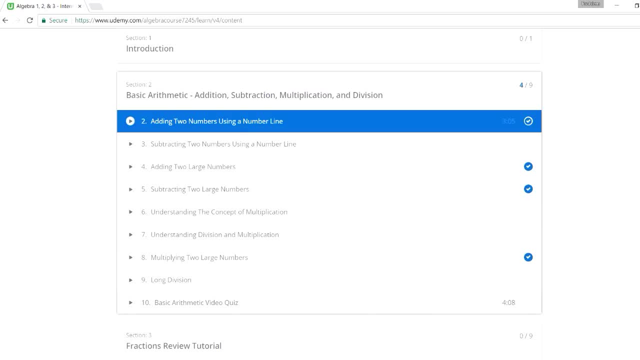 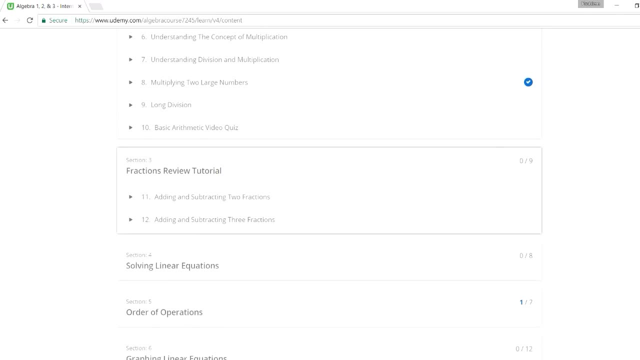 It's a multiple choice video quiz. You can pause it, work on the problems and see the solutions. It covers long division, multiplying two large numbers and things like that. The next tutorial is on fractions: Adding, subtracting, fractions. 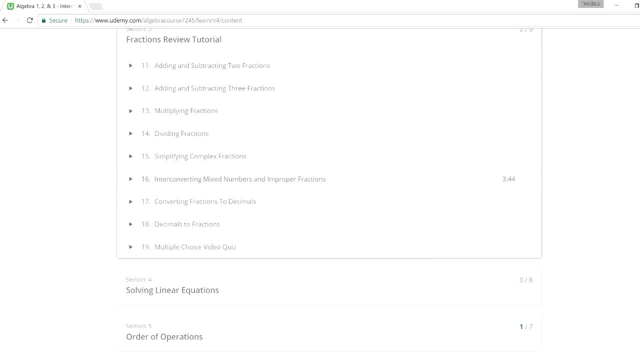 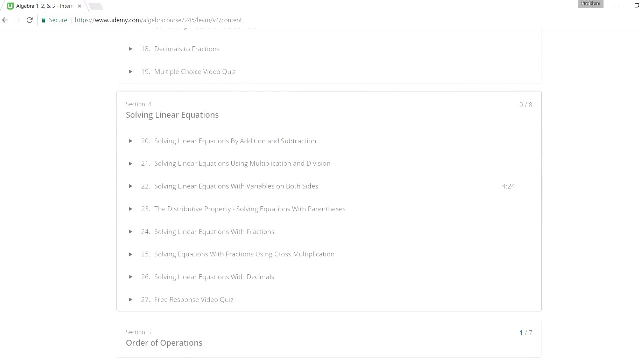 multiplying, dividing fractions, converting fractions into decimals and so forth. So you can also take a look at that. Next, solving linear equations, which we covered, And just more examples if you need more help with that. The next topic: order of operations. 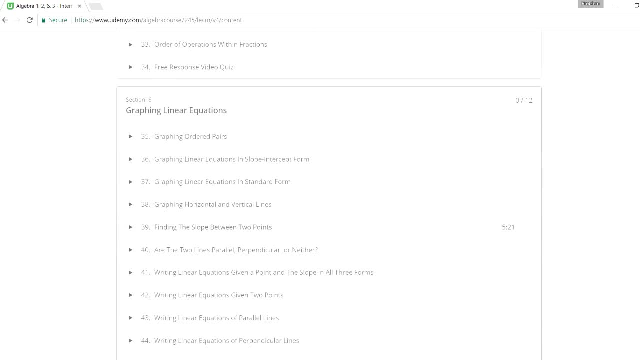 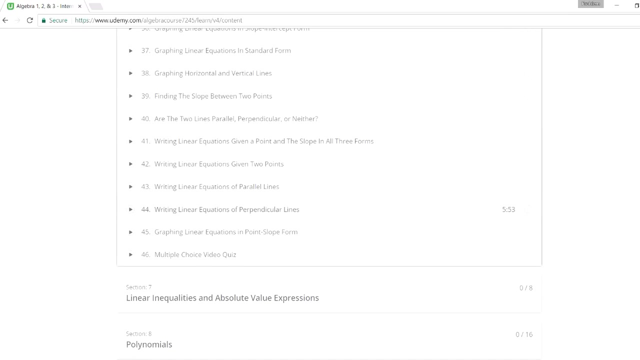 which is also useful Graphing linear equations. You need to know how to calculate the slope. You need to be familiar with the slope intercept form, standard form and just how to tell if lines are parallel, perpendicular and so forth. Use a quiz that goes with that as well. 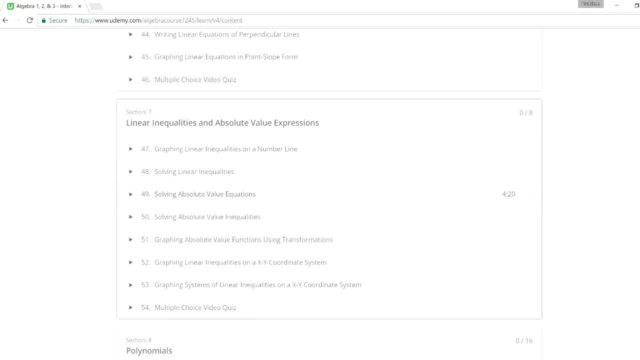 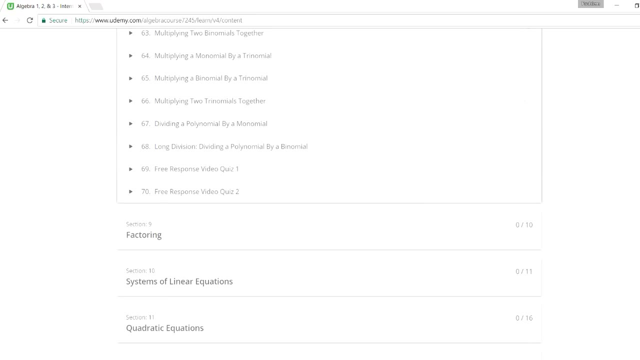 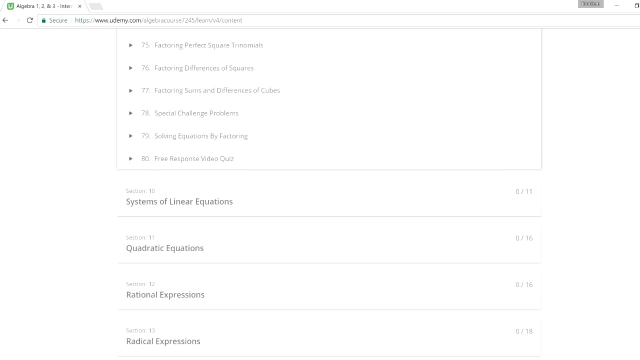 The next topic is on inequalities and absolute value expressions, which are also seen in a typical algebra course. And then we have polynomials, And that's a long section, And then factoring- That's another topic you need to master- And then system of equations.